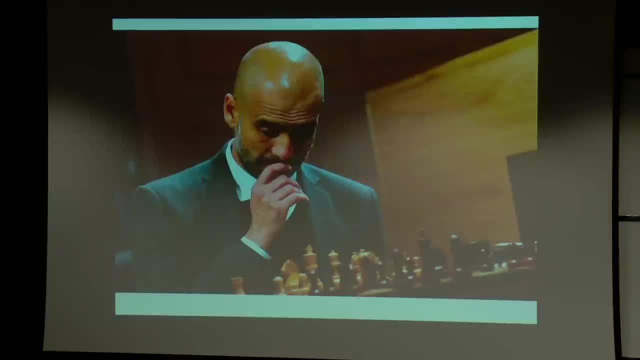 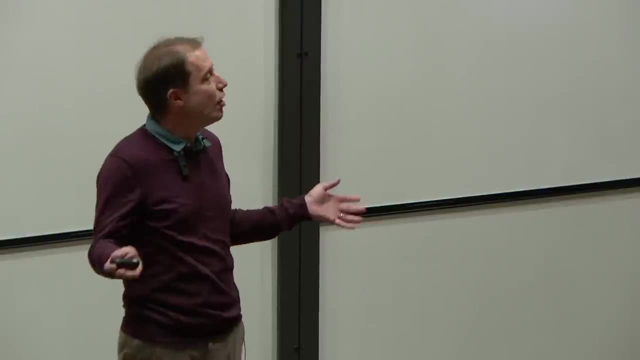 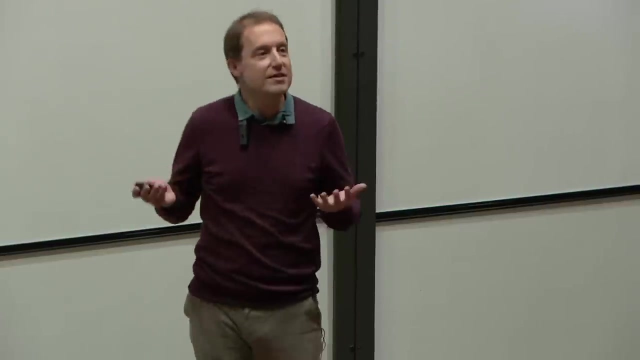 This is Pep Guardiola, And Guardiola. he's certainly passionate about the game, but he likes to sort of portray himself more as the kind of intellectual, the man who's opening up space for his team team and planning carefully about tactical decisions against the opposition. So there is. 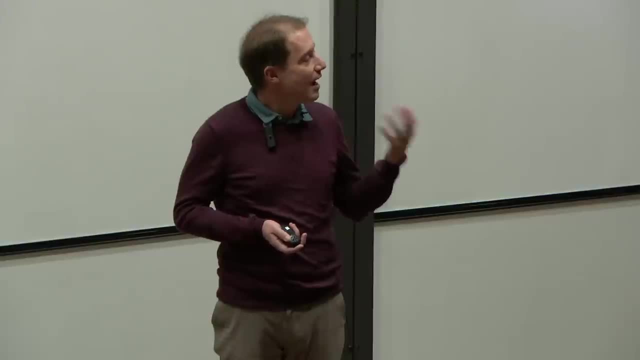 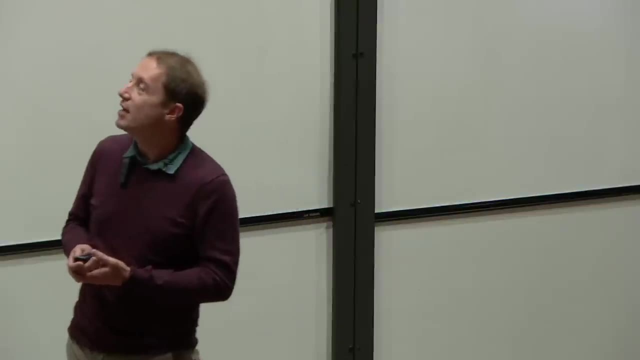 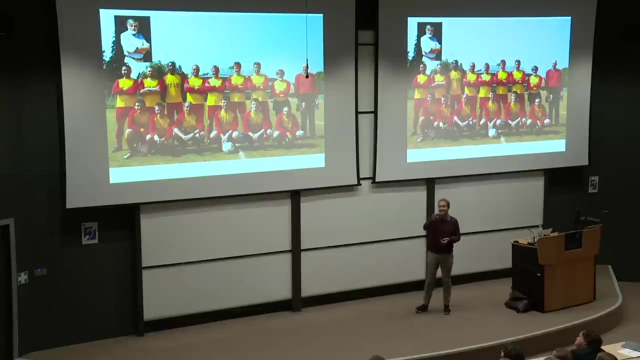 this kind of idea also of the football manager as the intellectual who's trying to solve a problem. And then there's also a type of mathematician, not the pure mathematician, but there's also the type of applied mathematician. And this brings us to Philip, who's sitting up there in the back row. 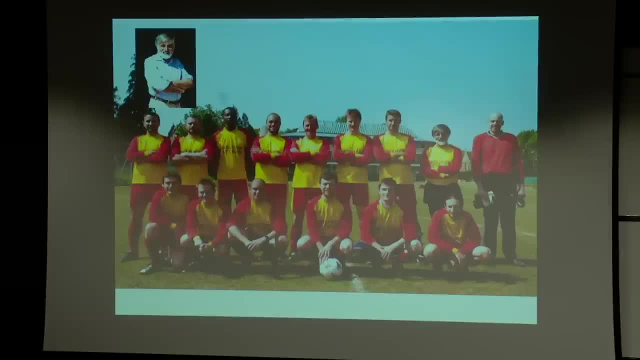 And this is Philip here And he's very kindly- this is the team he's been playing for- He's very kindly instructed the rest of the team exactly how you should stand when you have a photograph. You see, he's got his managerial style here And he's got most of them, seem to have. 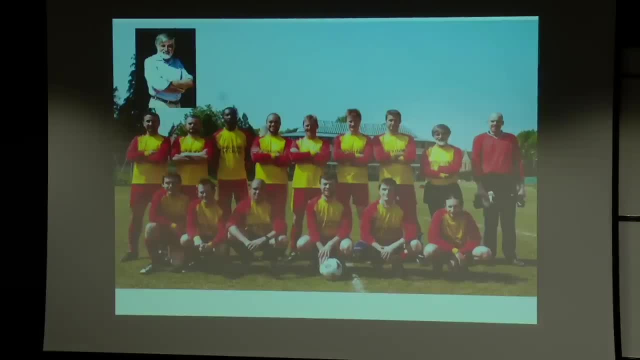 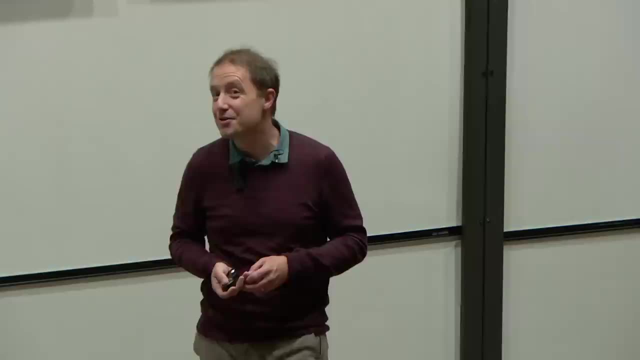 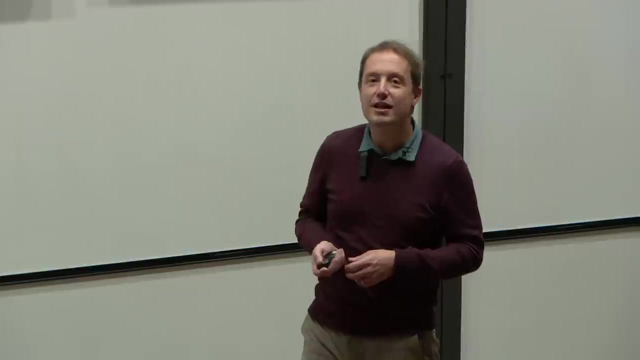 listened to his advice, And Philip is just one of several mathematicians who are accomplished football players. I don't know what league it was you played in, Philip. Can you tell us here? Okay, But we actually have another professor at Oxford who has played at a much higher level, So 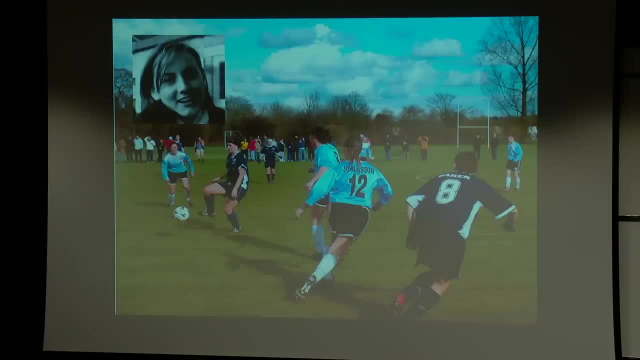 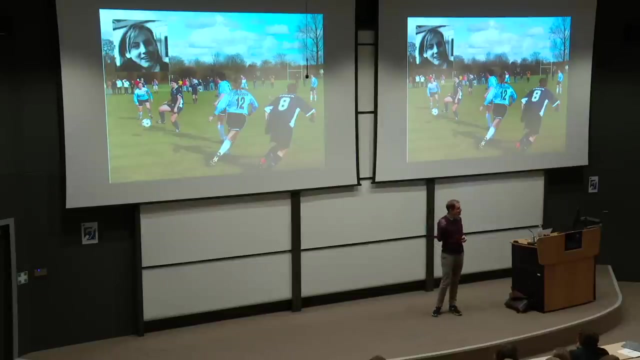 this is Ruth Baker, who's also professor of applied mathematics, mathematical biology, And she wears the number eight shirt, or has worn the number eight shirt for Oxford, So this must be a varsity. Where's Ruth? Okay, This must be a varsity match, And this was the one you won. 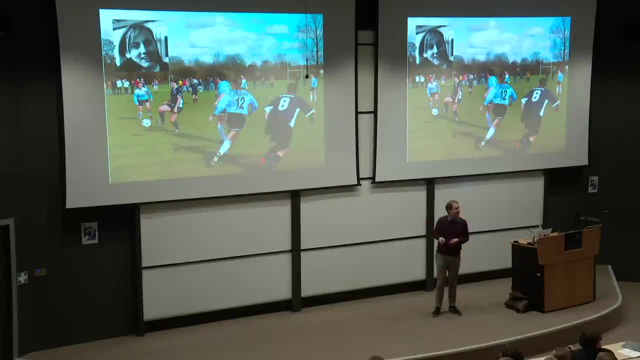 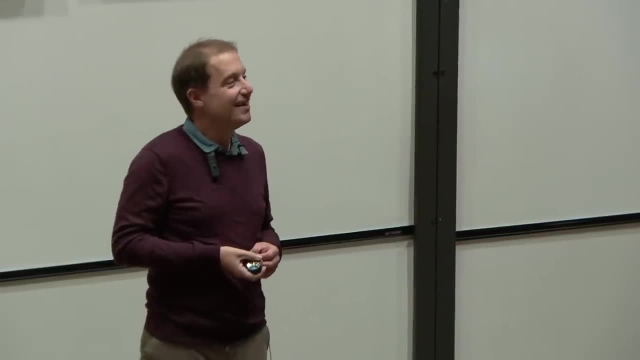 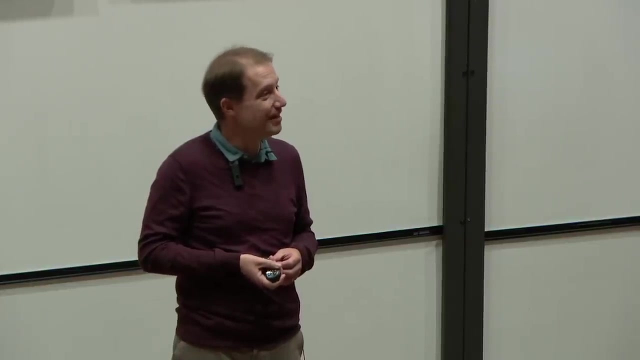 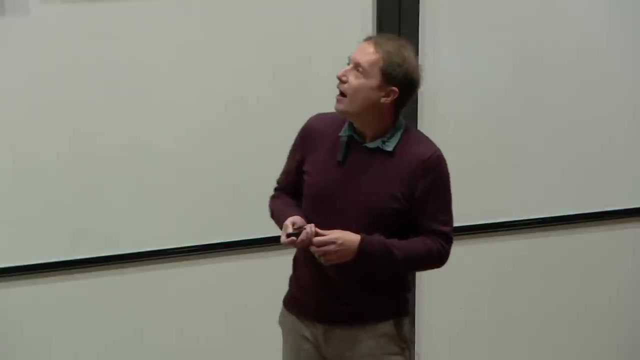 I take it. Yeah, Did you get the ball? You won that run, Can you remember? So it is possible to be a mathematician and to be a successful football player. You were described to me earlier today as the most successful football player in the whole Maths Institute. So very impressive. And I'm going to describe a little. 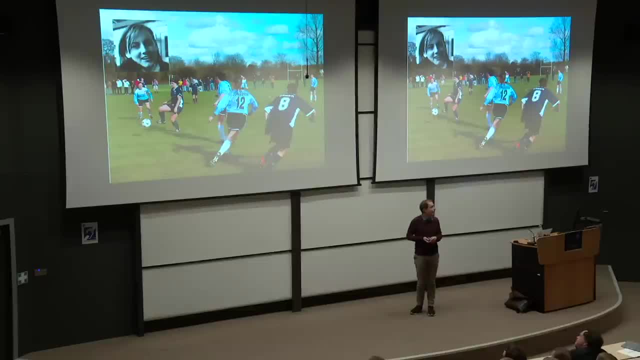 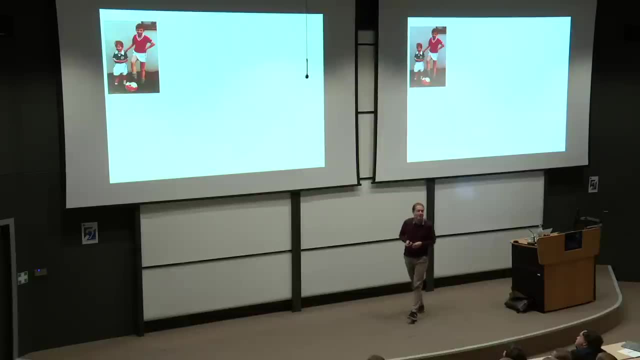 bit about my own background, So how I have gone from being a mathematician to becoming involved in football. I thought I'd start with a picture of myself when I was a kid. I'm, I'm the one, this one here, this cute one that's my little brother Colin. 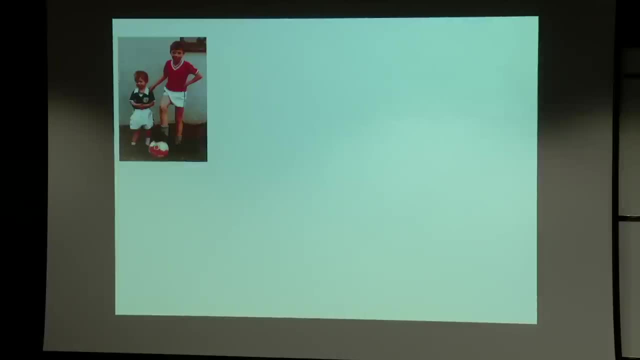 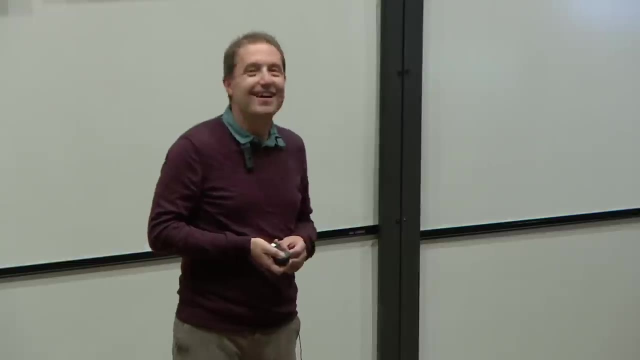 and this is me. I think I must have been about eight or nine when this photograph was taken and unfortunately I wasn't any good at football. I liked having the strip on and I thought I looked very good in it, but I found out that I wasn't. 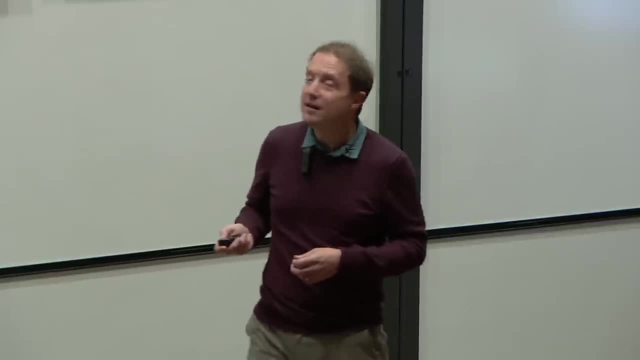 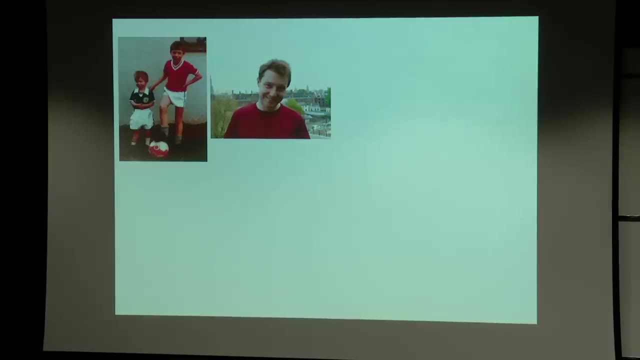 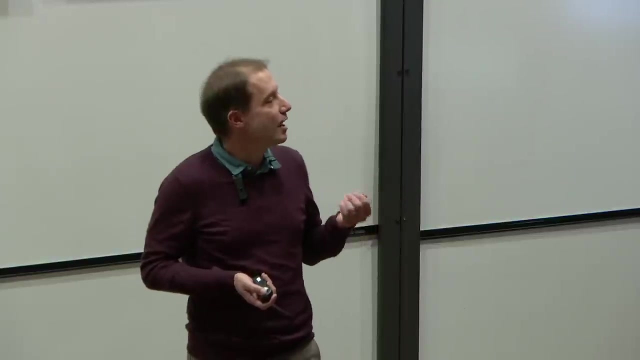 particularly talented football player, but what I was much better at was mathematics, and I have this picture of myself a few years later when I, as Alan said, I worked here as a Royal Society research fellow and I was particularly interested in one type of mathematics: how you could apply maths to understand. 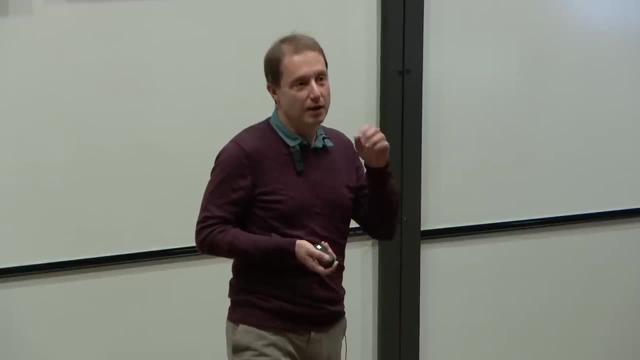 the real world and a lot of my research here. I was only half time based here at the maths department. I was also based at the zoology department and I worked together with people who were studying locusts, who were studying ants and pigeons. I think I have a picture of the pigeons here. these are actually. 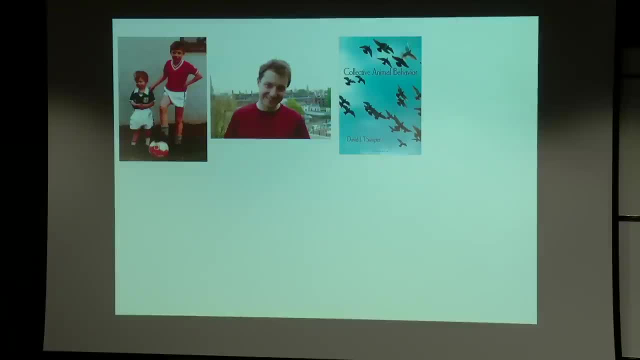 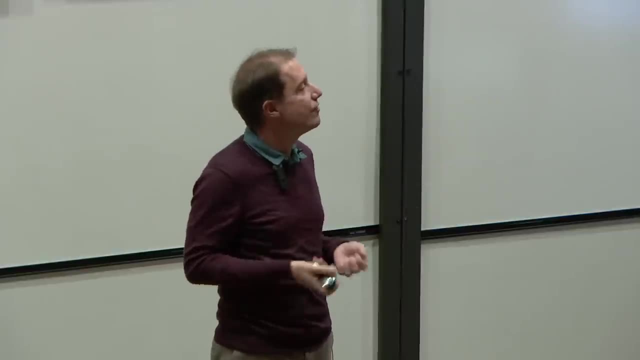 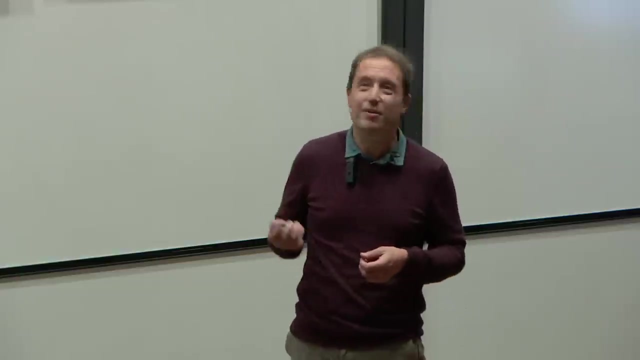 pigeons from from just outside Oxford. this was Dora Biro, who was one of my biologist colleagues who took this photographs, and I studied how they interact and how they produce different types of collective behavior. and oh yes, this gets on to the next picture, and I needed to put this in because I was at 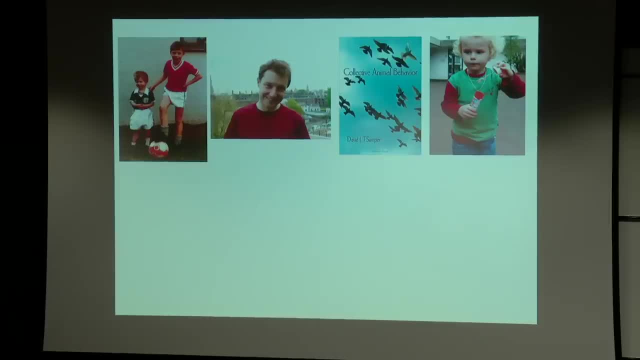 Wolfson College, and this is a picture of my daughter blowing bubbles in Wolfson College. I just wanted to have that in there as well, and then I became a professor in Uppsala, and then it turned out that my son Henry- who's this one here- he started. 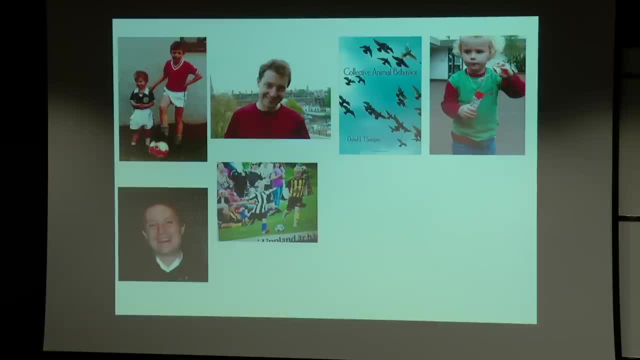 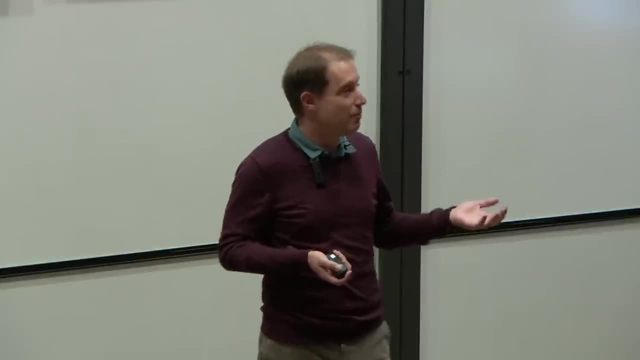 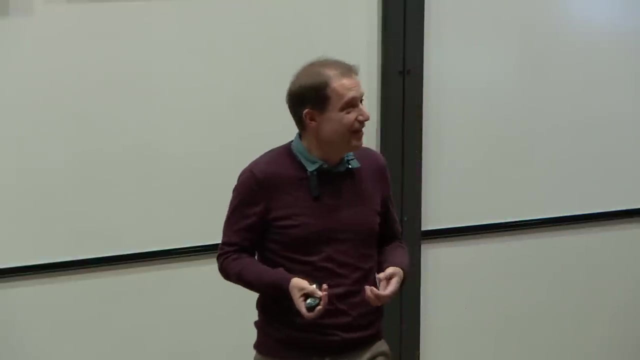 playing a lot of football and it turned out that he had a lot more talent at the game than I did and they needed people to manage his team. so I ended up partly with a bunch of other dads who were like overly enthusiastic, trying to relive their own failed dreams through their children. we started training as 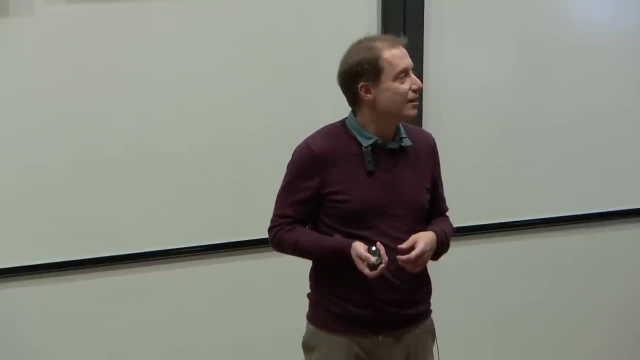 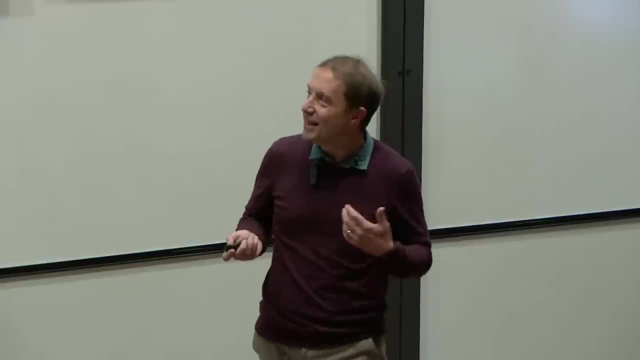 team and I'm still actually training his team. he's now 14 years old and he still still plays football on a regular basis. despite me embarrassing him in talks like this, he's still involved with it. and then I ended up because I became interested in football again and I'd always had that as it in a background. I 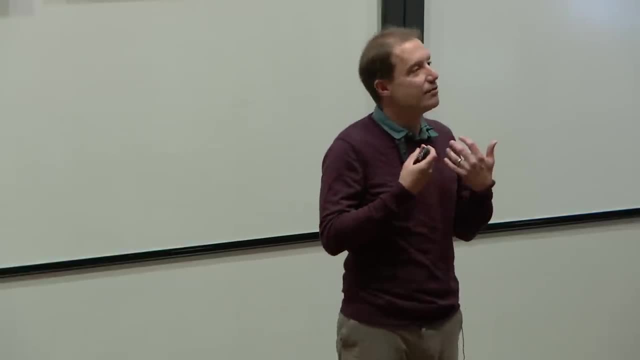 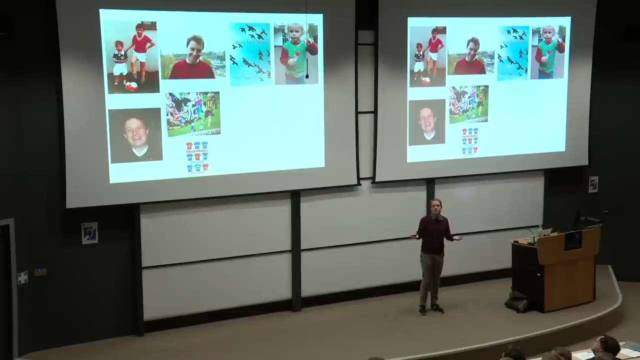 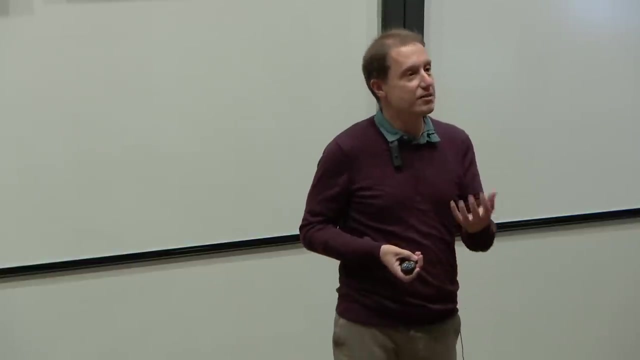 ended up writing the book Soccermatics, thinking about how we can use maths to explain different parts of football. and in the book I look at game theory for strategy. I look at randomness in the game, I look at passing networks- all aspects of mathematics that I knew I tried to bake down into the, into the. 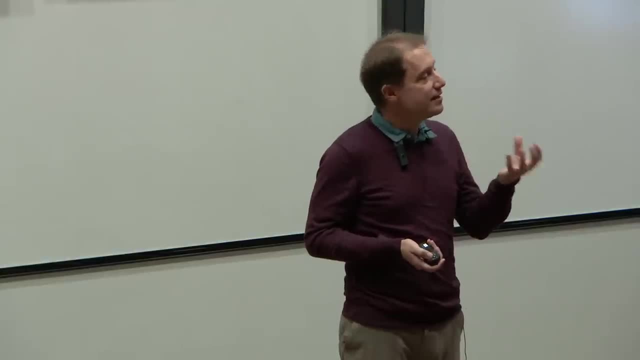 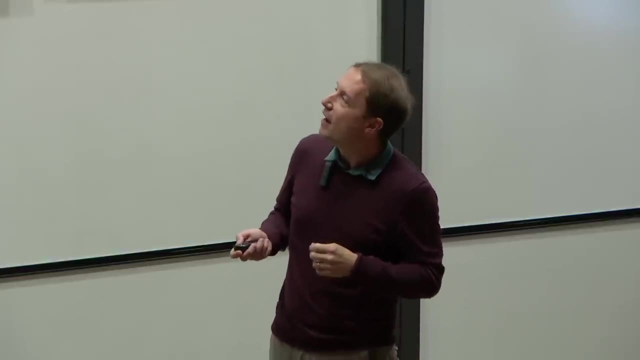 Soccermatics book, but this was mainly an academic. there was part of it was how you might apply it in reality, but it was mainly an academic exercise. and then I, as you get asked to do- you get asked to do a lot of things and I think it's. 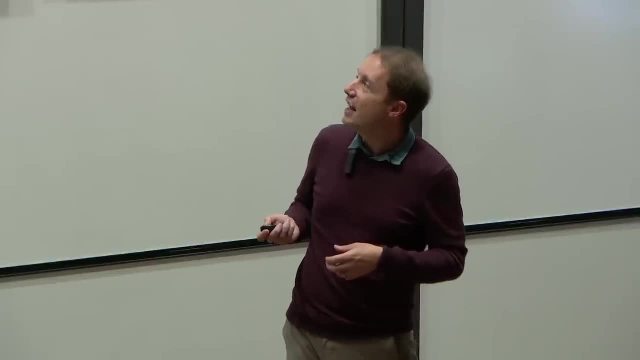 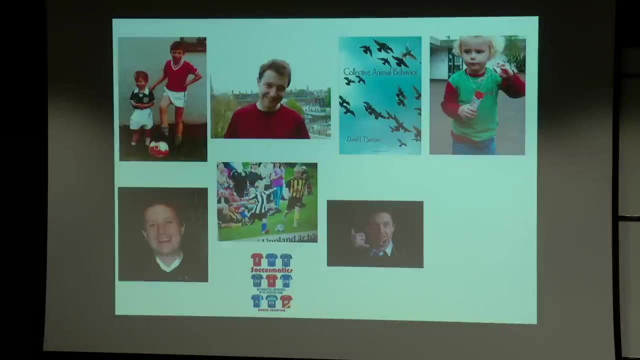 really important that you get asked to do kind of talks when you write a book like this. I got asked to do a TED talk and in that TED talk- or it was a TEDx talk- you should make a distinction here- but in that talk I put my hand up to. 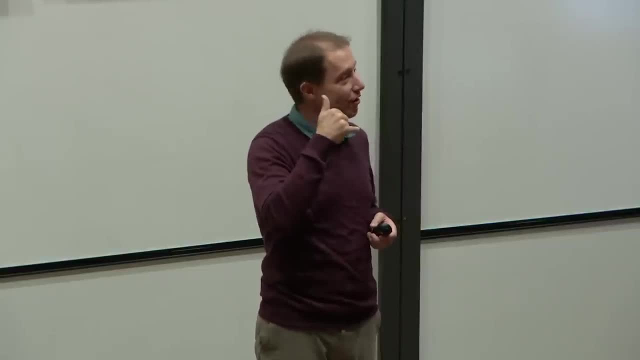 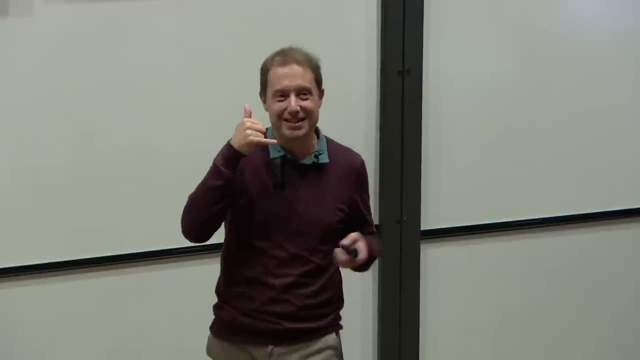 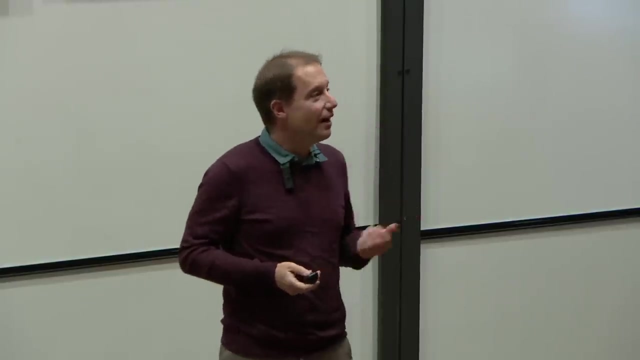 with a telephone and told Jurgen Klopp being a Liverpool fan. I told Jurgen Klopp: well, you know you can ring me anytime and I'll help Liverpool get promoted or win the Champions League or whatever. and he didn't call me. but strangely, actually quite a few other clubs did call me and I have had a. 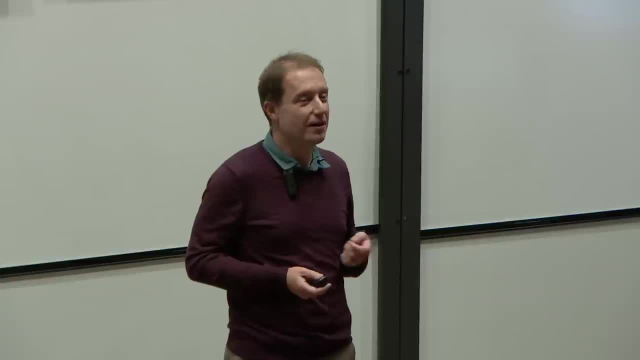 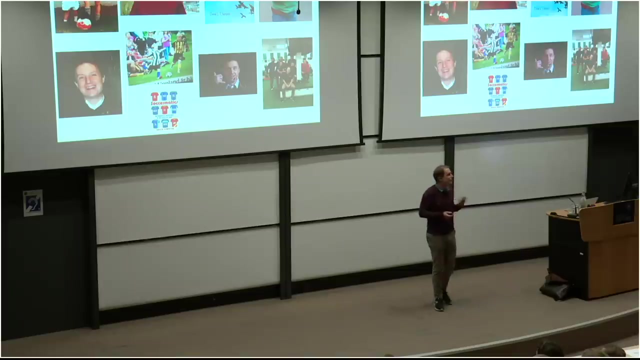 visit in Uppsala from two Premier League clubs. they made me write non-disclosure agreements, so I can't say which, and I've also visited a few clubs here in the UK- and another club that called me is the club Hammarby in in Stockholm- and they 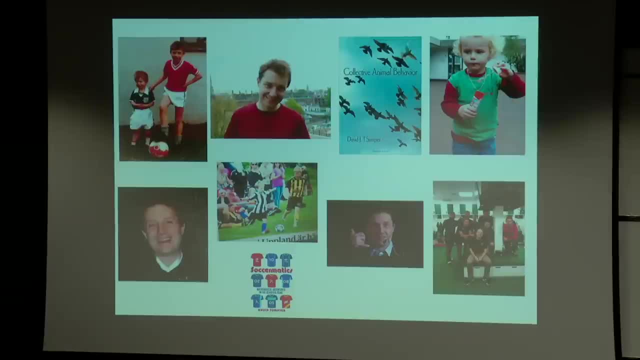 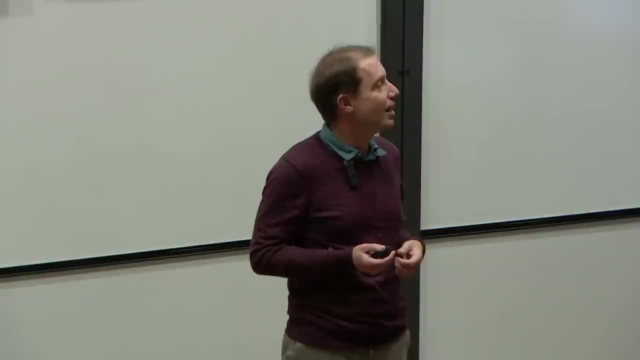 were very open and they said that I can actually go and work there, work together with coaches and with the players and help them develop their play with analytics, and so now I'm actually working part-time together with Hammarby Football Club trying to improve their game with mathematics. so that's a kind. 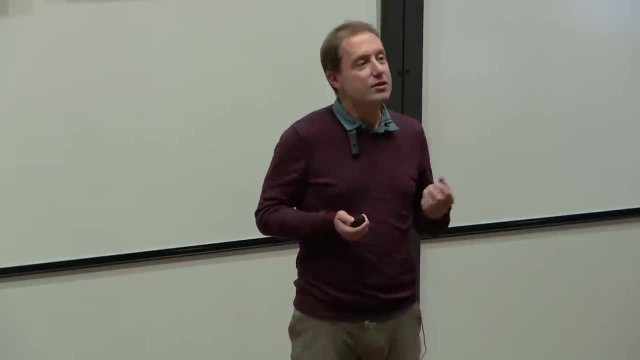 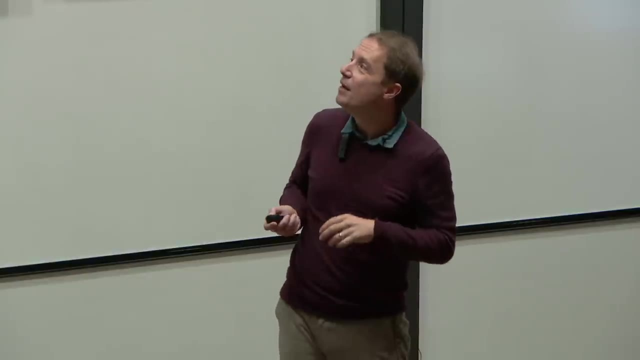 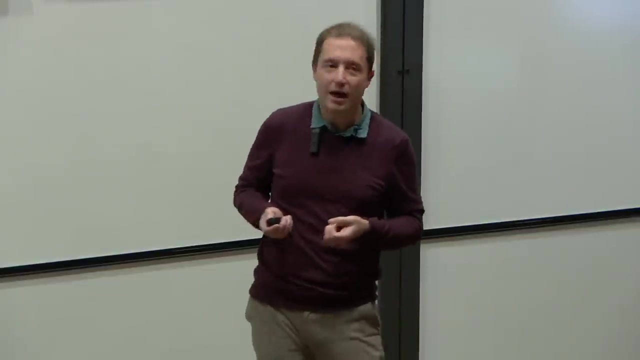 of brief history of of me, but what I'm now going to answer is: I don't think I'm quite there. I'm not actually managing Hammarby, I'm a long way from there- but what I want to get at is the basis of why applied mathematics is useful to a football team. 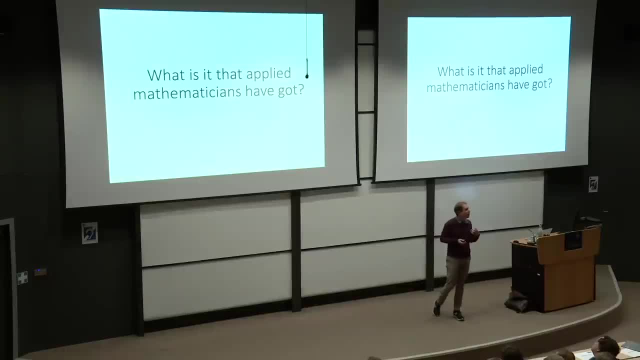 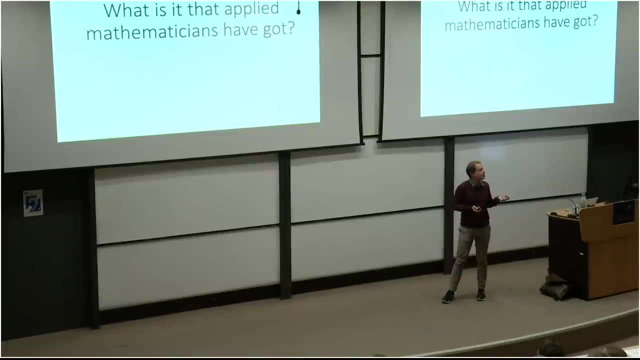 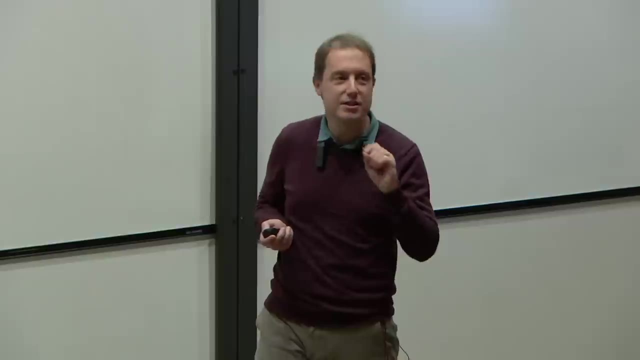 What is it that applied mathematicians have got that allows them to get somewhere in helping a football team? And I think I've been told that when you do a talk like this, you should be extremely clear what your message is, And so I've just written down precisely what my message is. 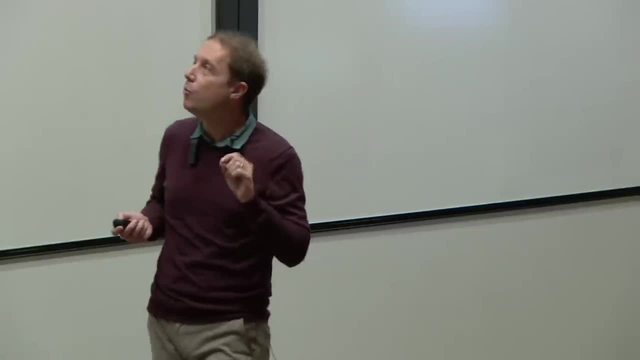 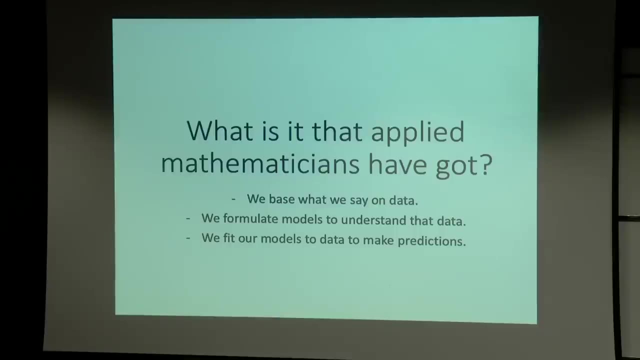 and I'm going to repeat it at the end of the talk: This is precisely what an applied mathematician has to give. We base what we say on data. When we talk about something, we collect data and we base what we see on data. 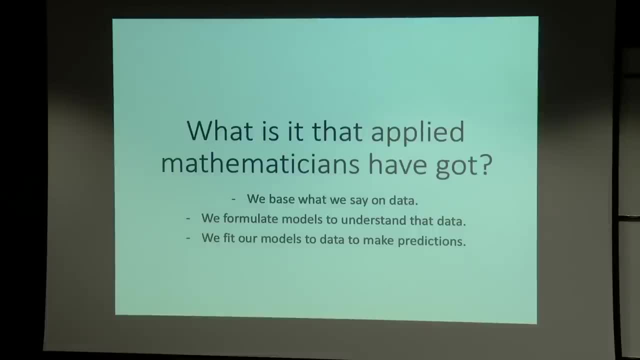 We formulate models to understand that data. It's an essential part of everything that we do that we have a model which describes how we think the data works and how we understand the data, And then we fit our models to the data in order to make predictions. 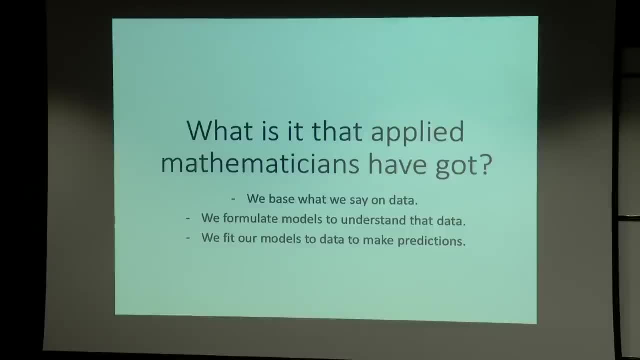 Predictions of the future. So that's the rules that we follow as applied mathematicians. What I'm going to spend the rest of the talk doing is explaining how we put this into practice exactly in football, And hopefully, by the end of it, I'll persuade you that. 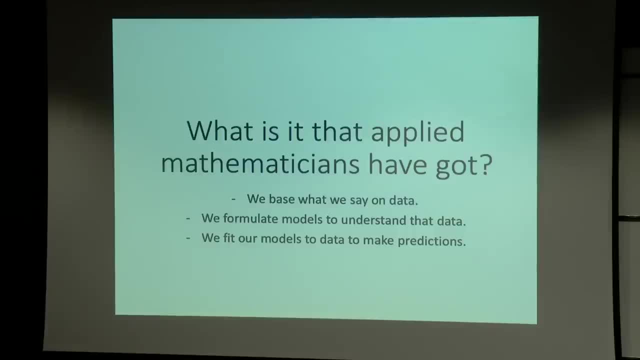 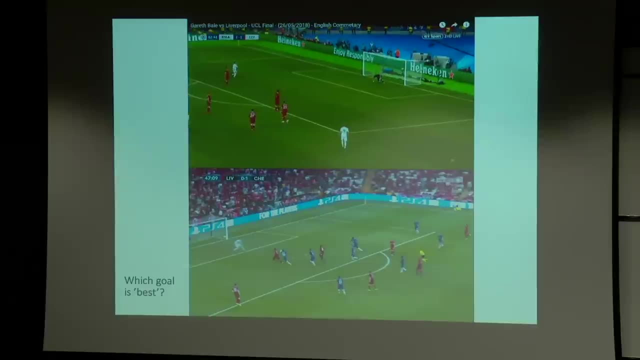 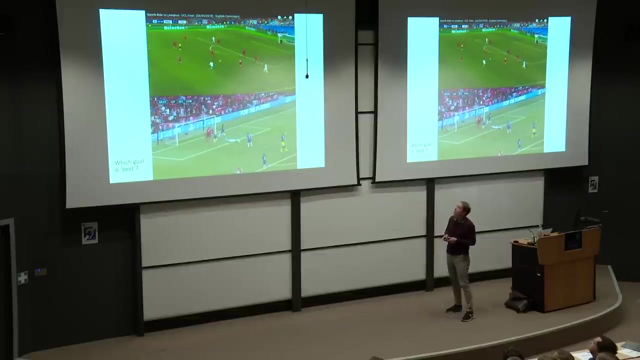 well, maybe applied mathematicians can be trusted to run a football team. So let me get to the base of this idea. right, Let's start with some goals, Goal. So I'm going to ask you a question. then, Out of these two goals, which do you think is the best goal? 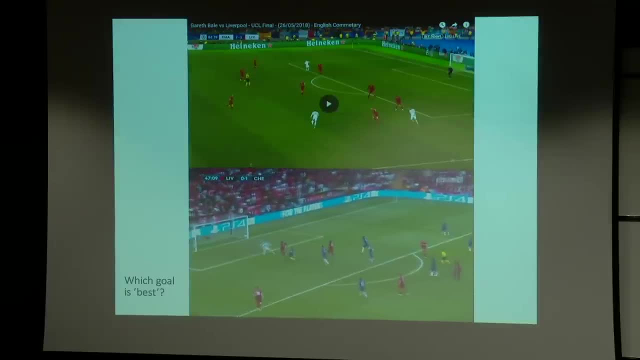 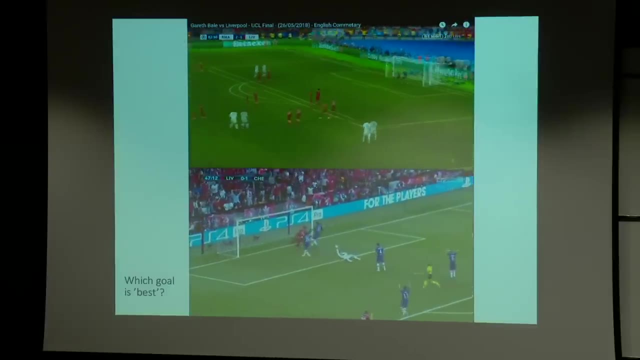 So let's put our hands up. Hands up for the top goal. Is that the best goal? And who thinks that the bottom one is the best goal? Okay, so we've got, I think, a slight majority for the top goal. 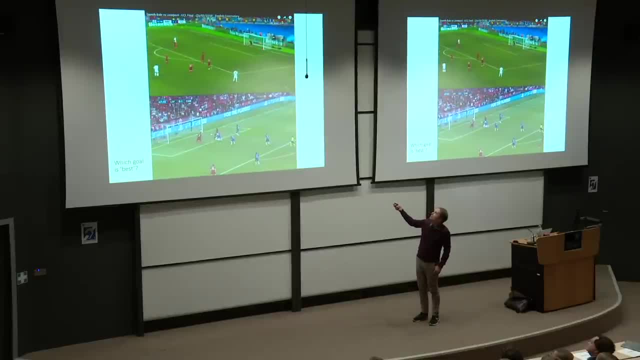 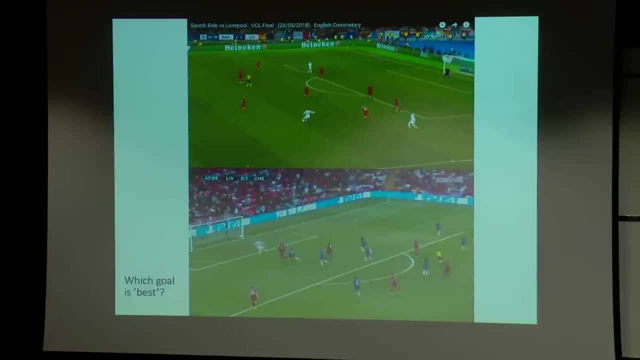 Now the top goal is a very long-distance shot. There is a mistake by the goalkeeper here letting it in. I don't like this goal. obviously, being a Liverpool fan, This was the reason we didn't win the Champions League last season. 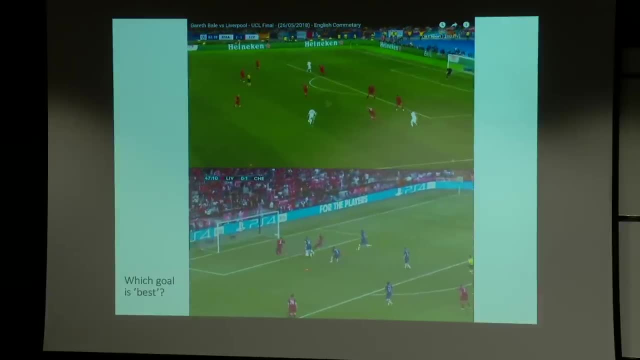 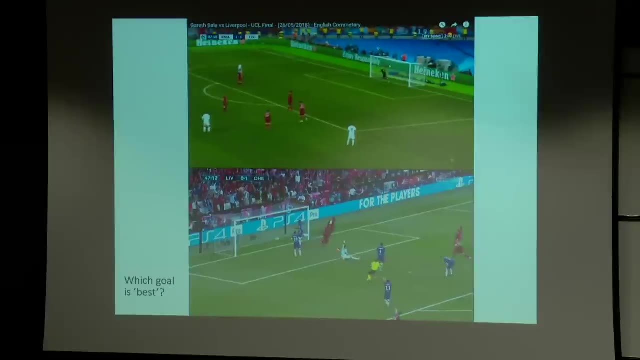 But the bottom one is a very, very messy goal. There's a lot of sort of things. There's a claim there by the goalkeeper that it was a foul- It clearly wasn't a foul- And the ball bumps into the back of the net. 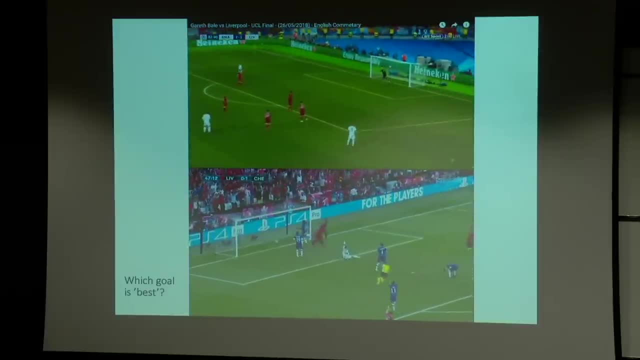 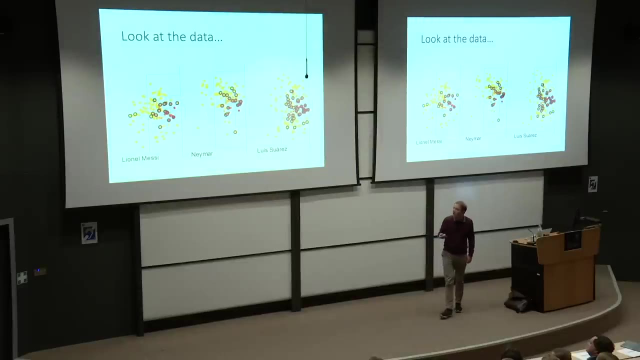 And so it's a much more messy type of goal. Well, what does maths have to say about this? Well, what we do is we start with this idea. We start by looking at the data, And now here is some data over lots and lots of goals in football matches. 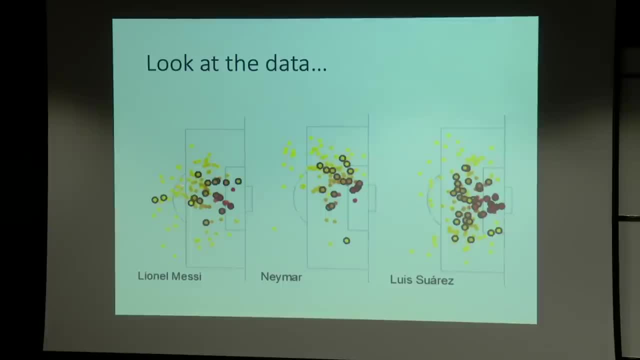 not just one. This is actually all of in a season of La Liga. this was the season before Neymar went to PSG. all of these little dots are shots that have been taken by these players: Lionel Messi, Neymar and Luis. 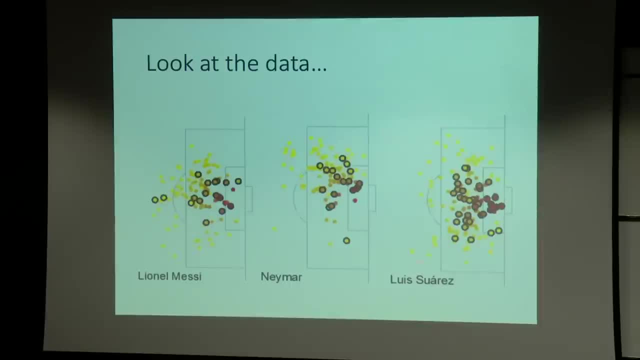 So this yellow is a shot from here. These are long-distance shots, And if there's a black circle around it, then that means that it was a goal. So this is where the goals were scored from And the important takeaway message from this. 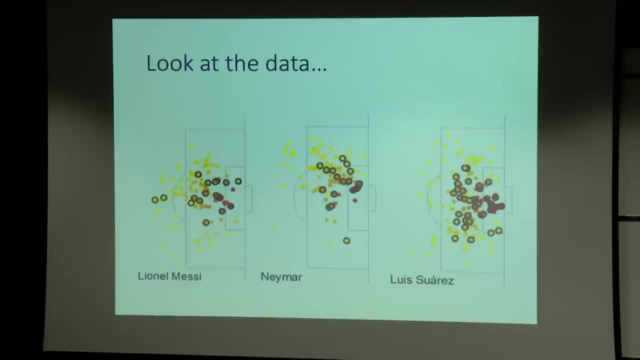 is that if you see where are the shots and where are the goals, nearly all of the goals are very close to the goal mouth. Even Neymar's are close. Messi has two which are slightly long-distance, But almost every goal that's scored by Barcelona in La Liga. 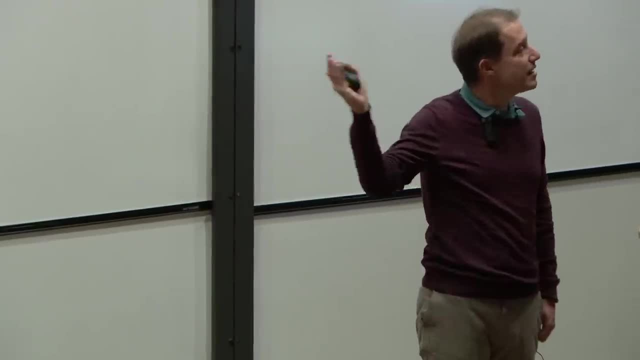 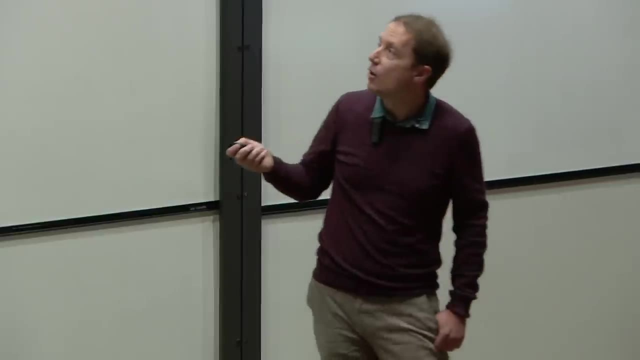 is scored very close to the goal, And that was exactly like Mane's goal at the bottom and not like Gareth Bale's goal at the top. So typically, goals are scored from much, much nearer to the goal. They're not scored at long-distance. 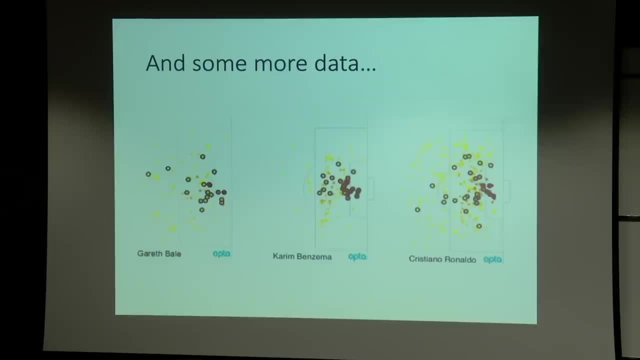 And this isn't just true of Barcelona. There are teams which shoot from a longer distance. This is for the same season. This is Real Madrid And Gareth Bale who scored the video. I think the goal in the video I showed you. 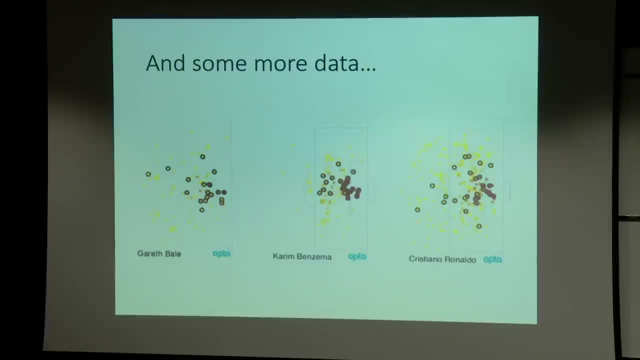 you see, he's got two long-distance goals, Cristiano Ronaldo. he has shot- I think it's- 60 times from outside the box and he's scored twice. So when he scores these goals and you often see them as the highlights on TV afterwards- 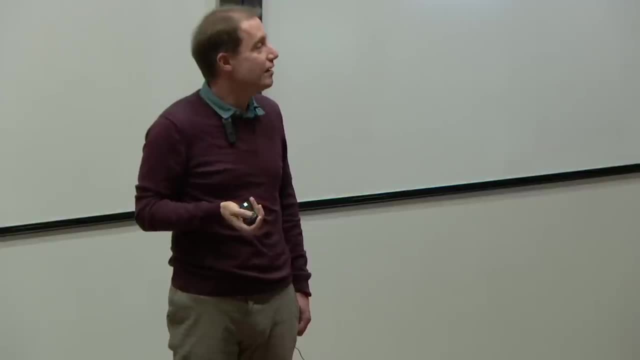 he actually scores only one out of 30 efforts, And you often see a YouTube compilation of all of the goals that he's scored. What they should really have in these goals, what they should really have in these YouTube compilations, is all of the misses that he's made. 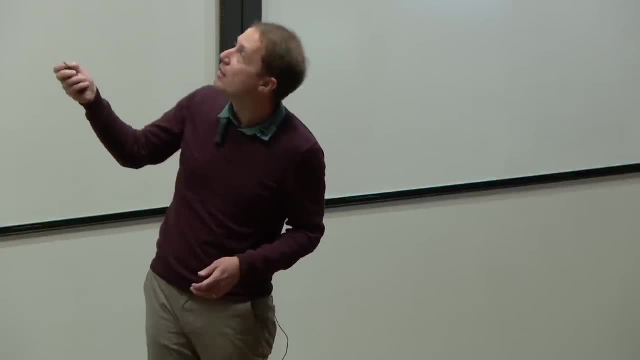 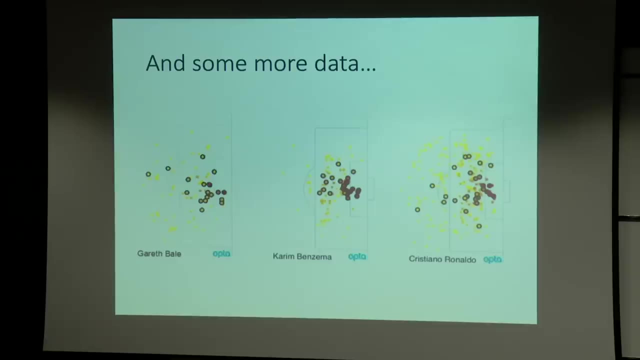 because he misses a lot of the time. Where Ronaldo scores a lot is actually very close to the goal. Most of his goals come from very nearby And that's our data. So we've got our data. Next step is the model, And I want to start. 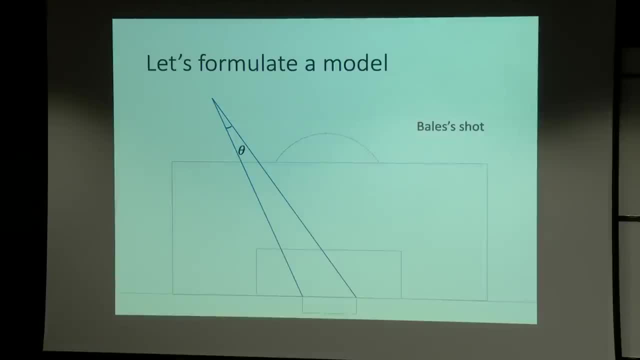 and I think this is always what applied mathematicians try to do. we start with the simplest possible model And then we build from there. And I want to start with the idea of this angle. And the angle is: how much of the face of the goal can you see? 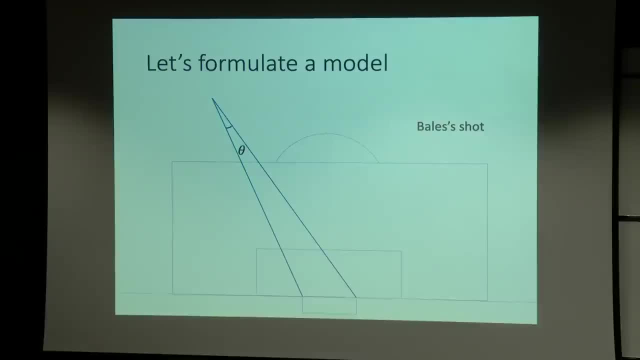 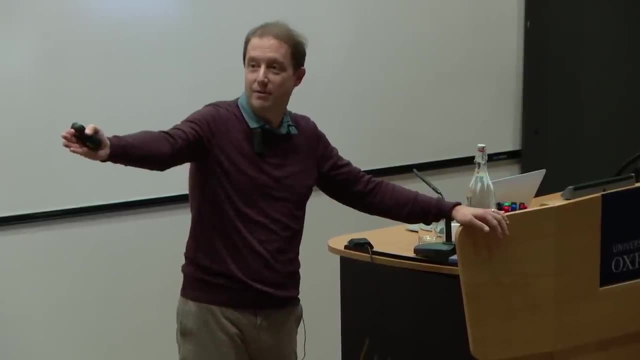 So, if you're looking, if we take this podium, for example, the people who are sitting straight on at that podium can see it much more clearly than the people who are sitting there. There's a much wider angle. The people who are sitting at the back. 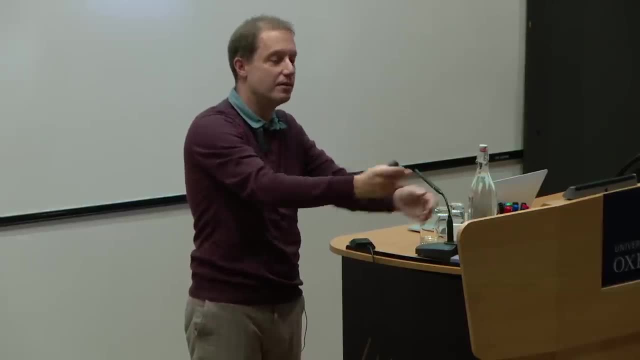 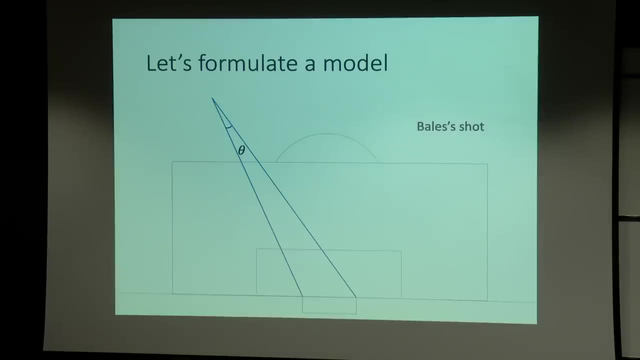 they have a narrower angle than the people who are sitting at the front, And so our basic idea is this angle to the goal post is going to be the model of the probability that you can score. Bale's shot is a long way out. 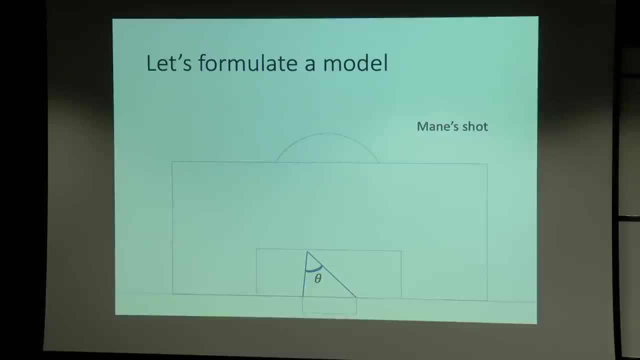 so it has a little angle. Manet's shot is very close in, so it has a very large angle, And so the quality of a chance in football can be assessed by the angle to the goal mouth here. And then you have this nice property that 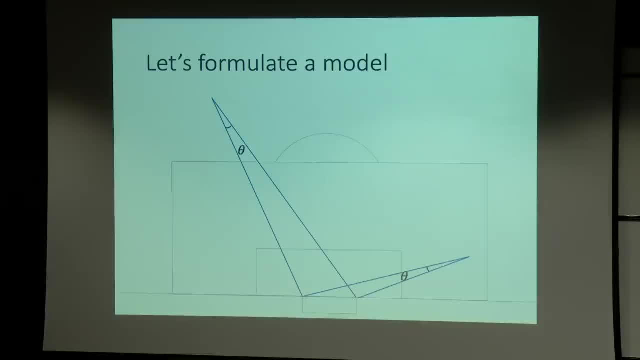 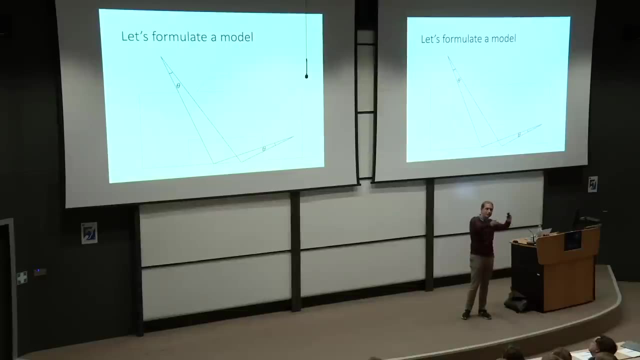 well, you can go around, as I mentioned that. people sitting out there looking at this, they have a very narrow angle even though they're closer to me. But people sitting up there, they might have a similar somewhere around there. 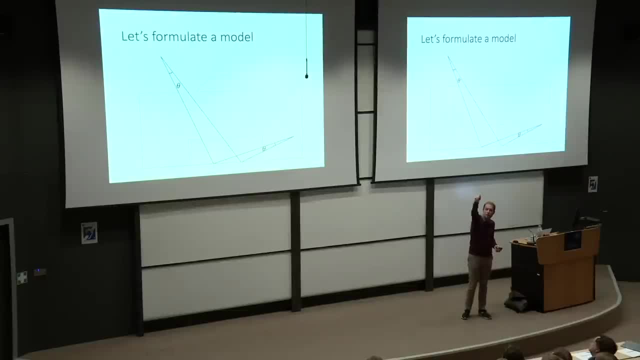 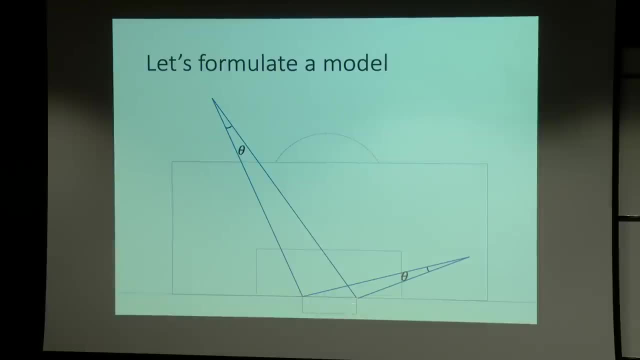 they would have a similar angle And there's actually a circle which stretches out from the goal. All of those points on the circle are: this is a segment of the circle here and there's a circle that goes all the way around and all of those points are on the circle. 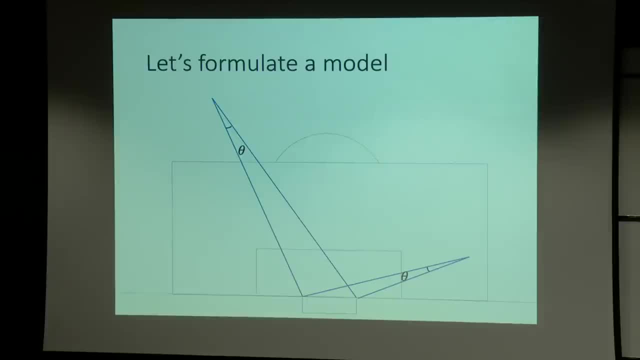 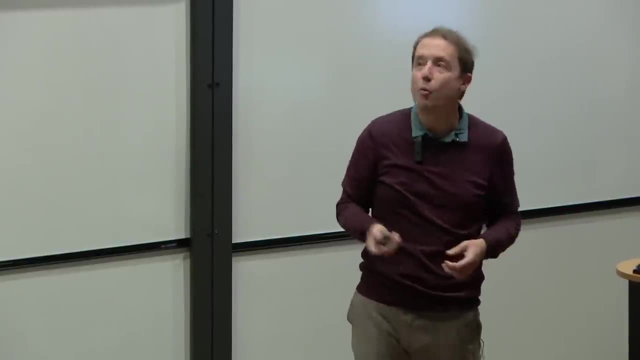 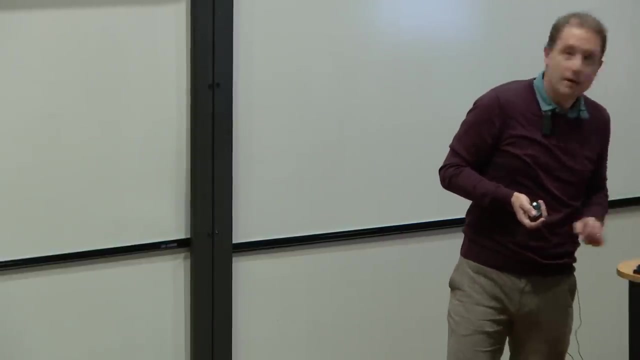 And so now we can define basically- this is the essential bit here of applied mathematics. Applied mathematicians are always going on about how many parameters they have in their model. Here we just have a one parameter model, this angle, which defines the probability of scoring. 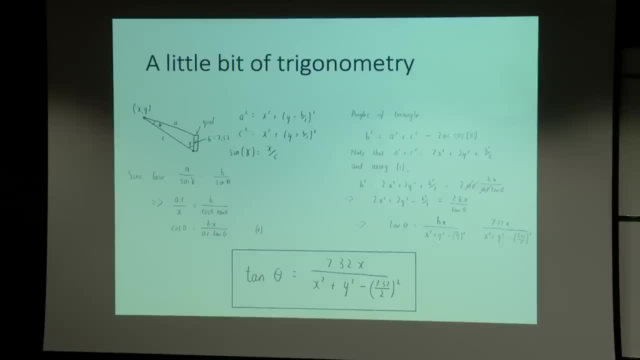 A little bit of trigonometry. This is something I did by hand. You can actually work out from the xy coordinates of the shot. you can work out the angle. I won't go through the calculation, but you end up finding that these circles 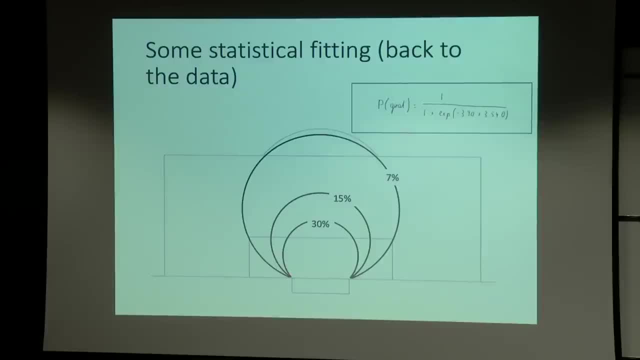 all have exactly the same angle, and now the next thing we're going to do is we're going to actually take data into this, And what we do is we do a thing called logistic regression, where we take all of the shots that have been taken. 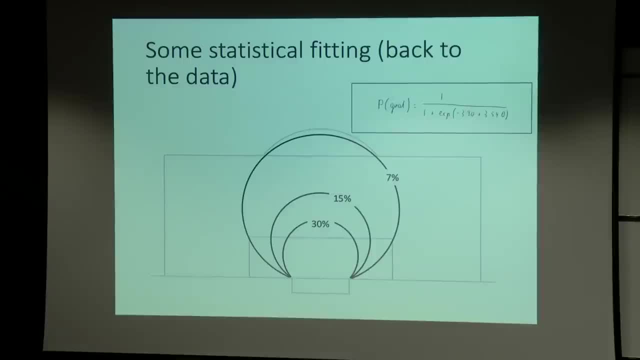 in La Liga or in the Premier League and we calculate the angle for them and we calculate using logistic regression. we calculate the probability of them scoring a goal as a function of this angle And by computer fitting I get these two parameters. 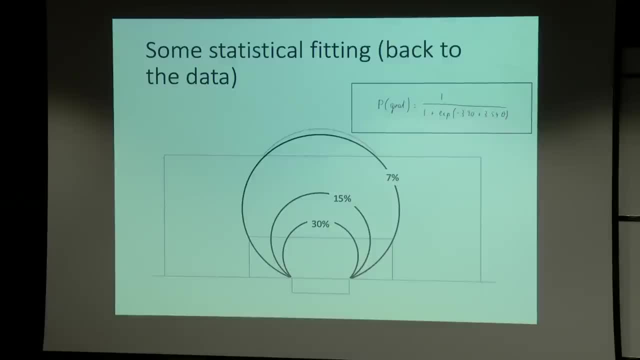 3.54 times the angle theta, and then this constant here And they can then tell us the probability of scoring from different angles. It turns out the one parameter model isn't perfect. It turns out you do need to actually put in the x coordinate. 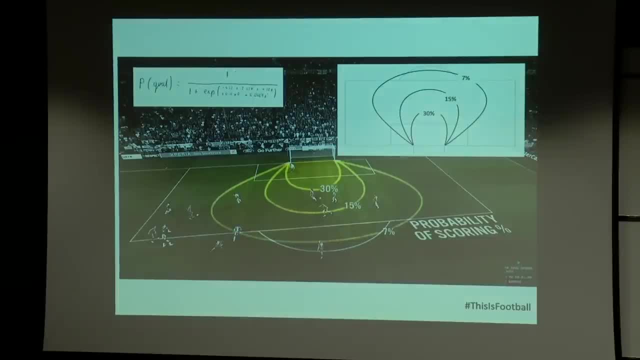 to get the best fit to this data. But this roughly gives a universal rule for scoring in football that there is a 30% chance here, a 15% chance here and then there's a 7% chance out in this circle. 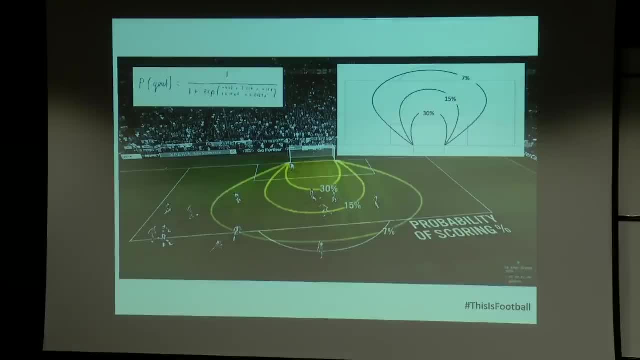 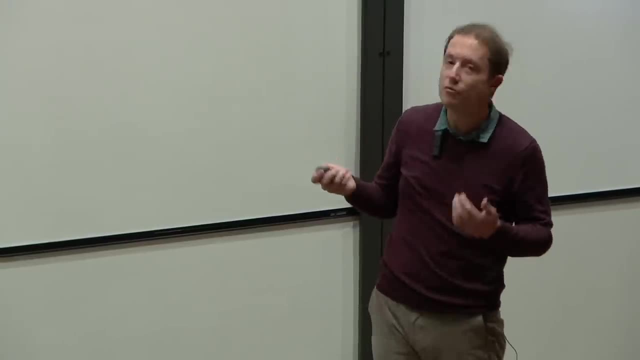 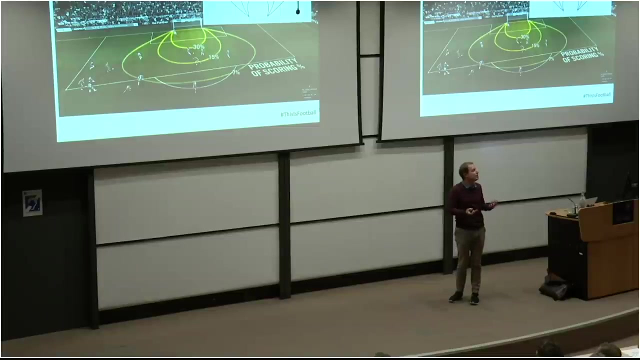 And that's roughly true across a wide range of leagues. And if you have looked at things like football analytics, which there's lots of, this is the basis of what's called the expected goals model. Basically, this probability gives the probability on an average day of football. 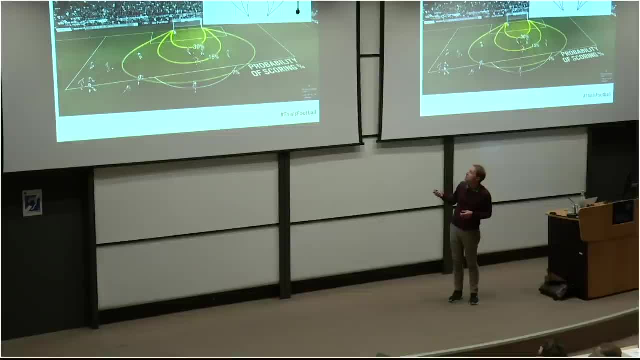 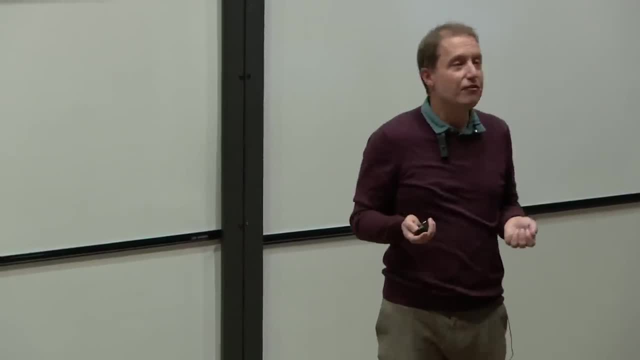 that you'll score a goal in these different situations. So it's called the expected goals model And it works very well. It turns out the teams that have the best expected goals in the long term they do well, And so this is an example. 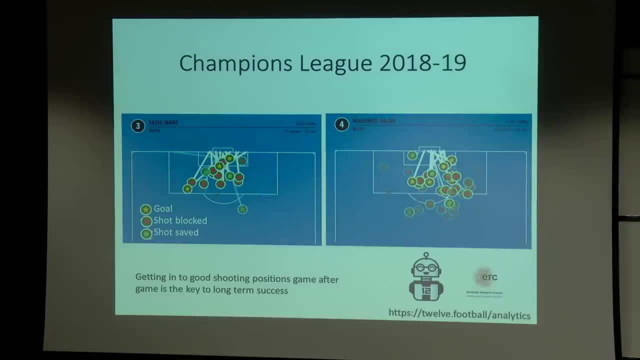 There's an online app If you want to go in and look at your team's expected goals. it works for the Premier League, for the last few seasons, the Champions League and so on. You can go into our 12 football analytics app. 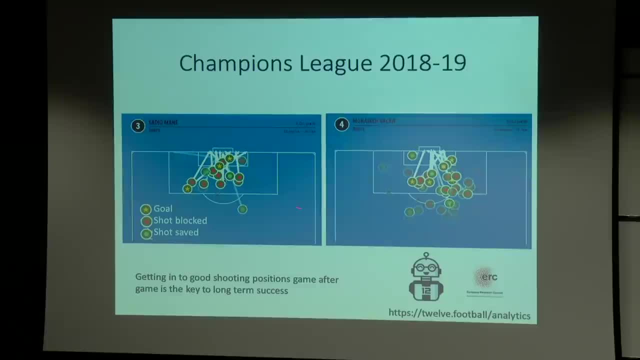 and you can actually look at the shots that the players have got. And here you see why Liverpool won the Champions League. Mane took so many shots from very close to the goal. Lots of them were misses, but lots of them were goals And the same thing. 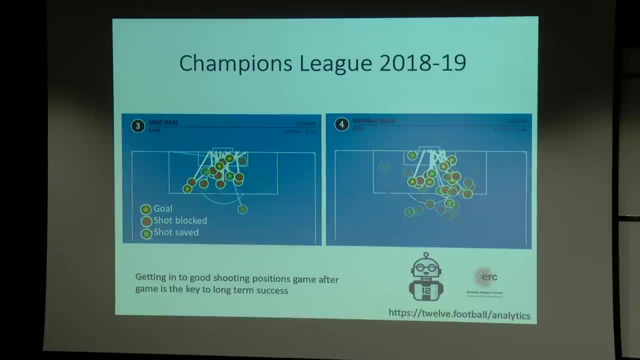 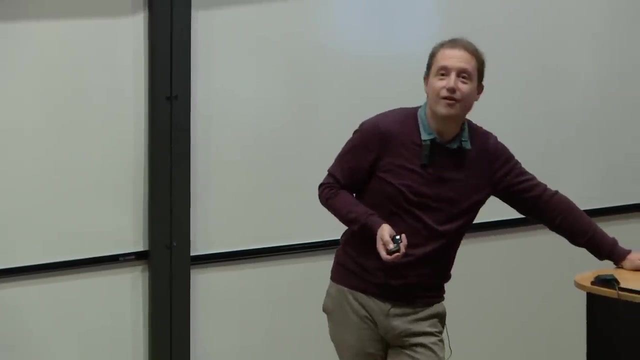 with Mohamed Salah, So they've specialised in getting extremely close to the goal before they shoot, getting inside those circles and producing a lot of goals as a result. I've got something similar for Ronaldo. Now I've got one more thing here for Philip. 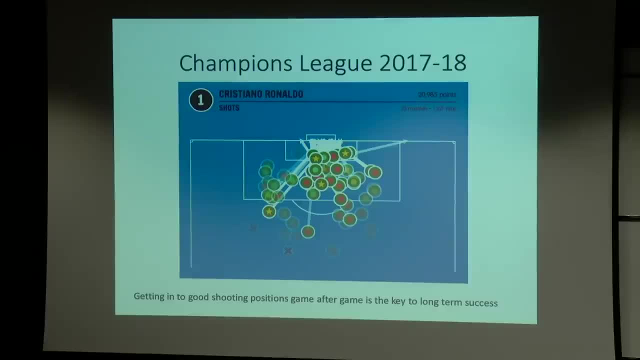 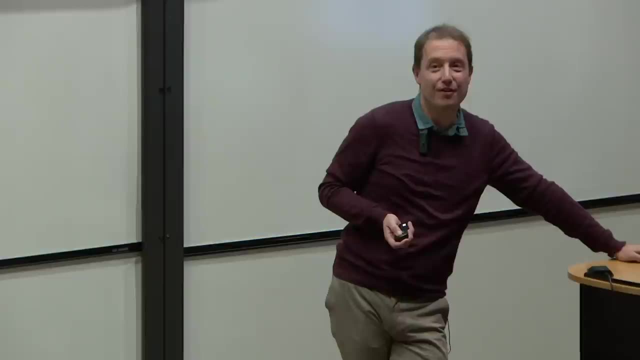 who's a Leeds United fan If you use this measure, Leeds United- last season they failed to qualify for the Champions League for the Premiership, But it turns out when I calculated, or when Opta calculated, the expected goals for Leeds United, it turns out. 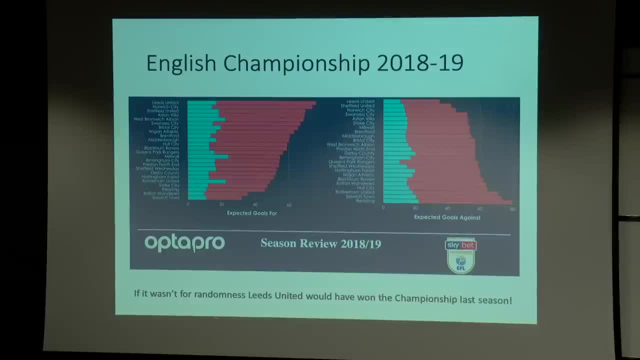 they were extremely unlucky. If it wasn't for randomness, Leeds United would have won the Championship last season. If you look at this chart, they scored more expected goals, had better chances than any other team. They conceded fewer chances than any other team. 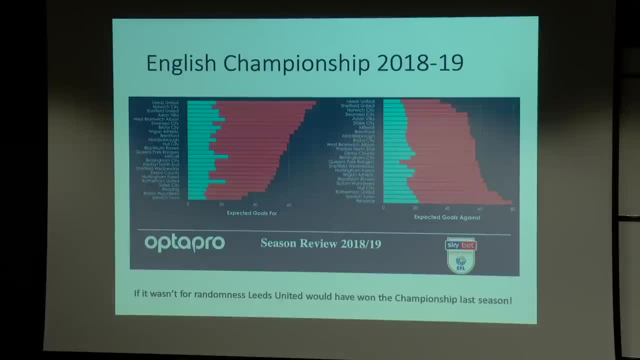 but they still weren't promoted. So there's a lot of unfair randomness in football That we can't really get away from, But we can get an overall underlying idea of how good teams are, And Leeds United are actually doing it very well this season again. 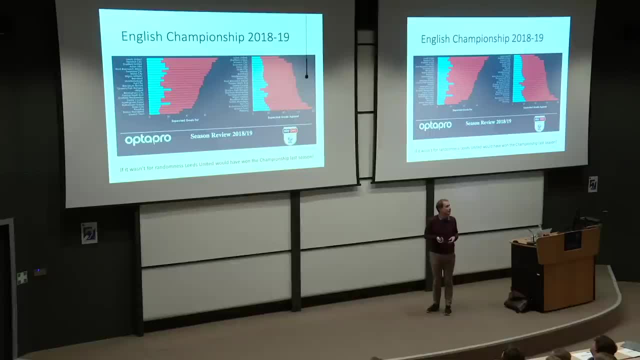 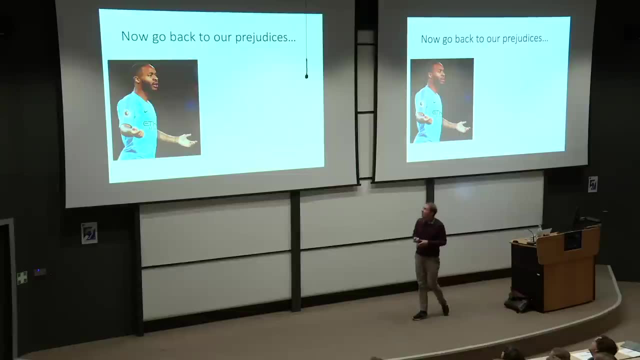 So I think that they, because they're good in this measure, they will eventually, if they can keep it up, get promoted OK. so I want to go back to some of our prejudices, because I think what's very interesting when you've got 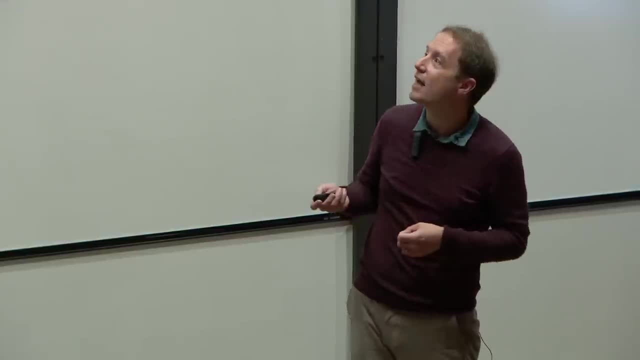 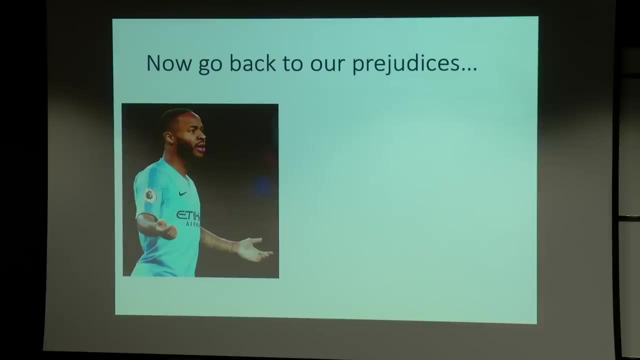 a statistical tool like this or a mathematical tool for understanding the world, how can you use it? Well, one way you can use it is the following. So this is Raheem Sterling. He plays for Manchester City And this is the type of headline. 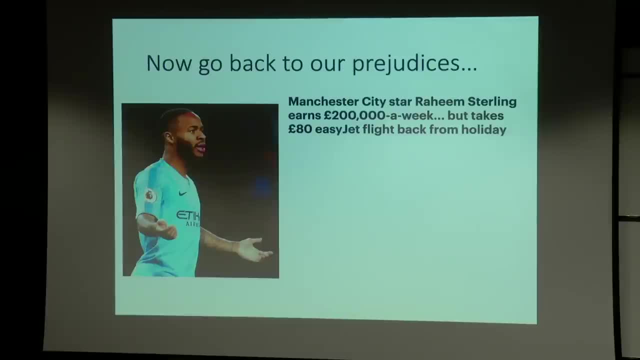 that you see about Raheem Sterling in certain newspapers. This is a headline from the Daily Mail. Manchester City star Raheem Sterling earns 200,000 a week but takes an 80 pound easy jet flight. Apparently, this is somehow really bad behaviour. on the part of Raheem Sterling. How dare he take an easy jet flight? But even worse, the Sun found out that Raheem Sterling, he hired a private jet and headed out for two holidays in a week. So Raheem Sterling can't win. 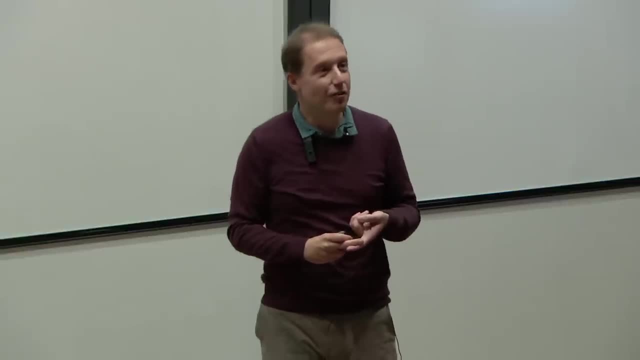 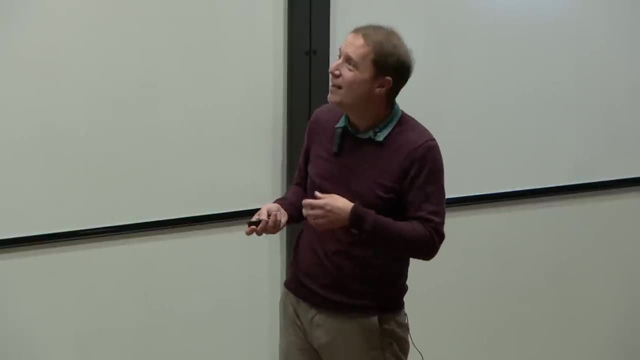 If he goes on a cheap, easy jet flight, that's really bad. You know, cheap football player, he earns so much money. But if he hires a private jet, then there's something wrong about that, And what you'll often hear is this sort of justification. 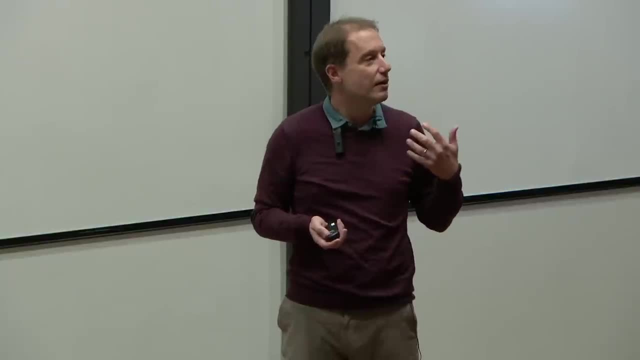 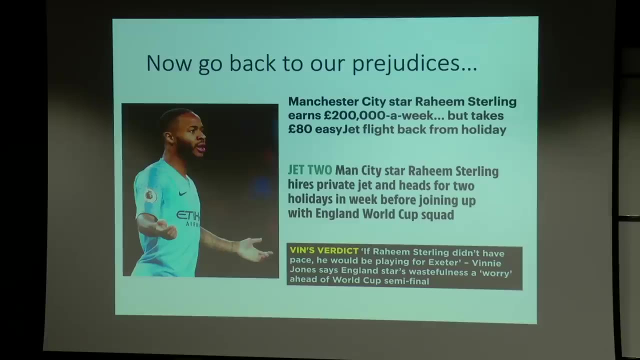 of why they say bad things about Raheem Sterling is that he's not playing very well or he's not doing all he can for the team that he plays for. And Vinnie Jones came out and said: if Raheem Sterling didn't have pace, 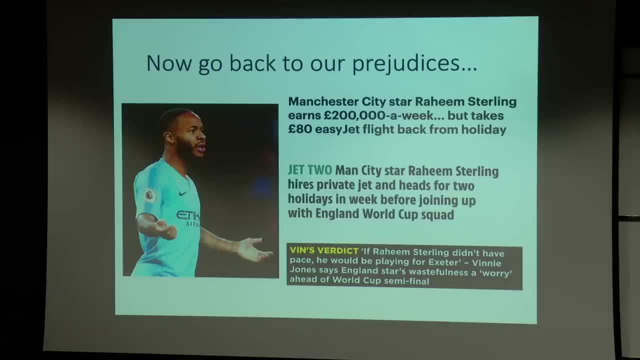 he would be playing for Exeter And Vinnie Jones. so, despite the fact that they got to the semi- the semi-final of the World Cup, with Raheem Sterling playing in every match, Vinnie Jones was worried that he was wasting too many chances. 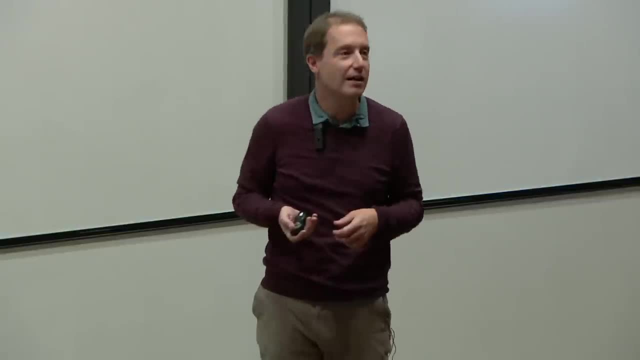 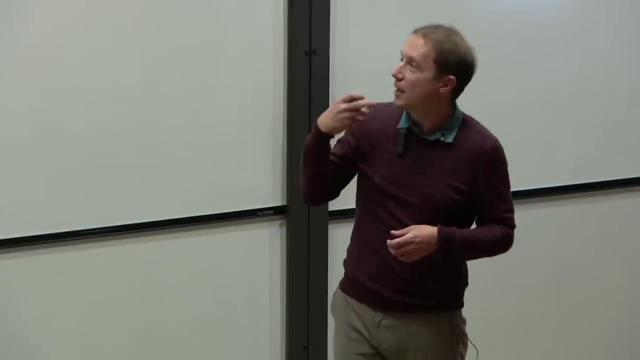 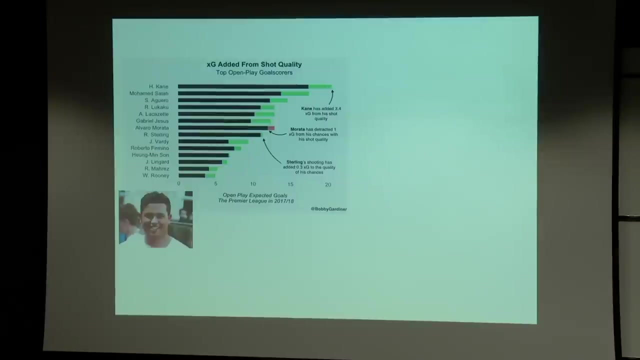 So Raheem was to blame, And so you get these types of headlines about players all the time. And what a colleague or another person who's interested in football analytics- Bobby Gardner- did? is he actually studied this? statistically? Is Raheem Sterling? 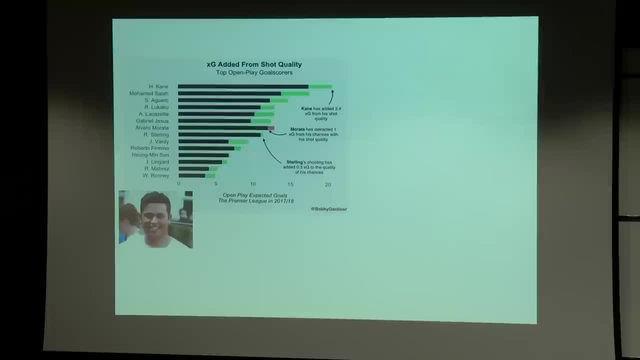 wasting lots of chances, like Vinnie Jones says, And it turns out he isn't. If you compare his expected goals with his actual goals, he's spot on. So the chances that he gets he converts as an average striker or a top-level striker would. 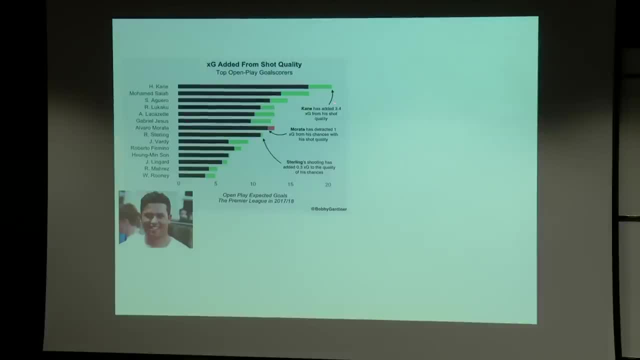 So you have people who overperform, For example, Harry Kane overperforms, Mohamed Salah overperforms, But Raheem Sterling plays out on the left. He isn't their top striker. That's actually Aguero who's up there on the list. 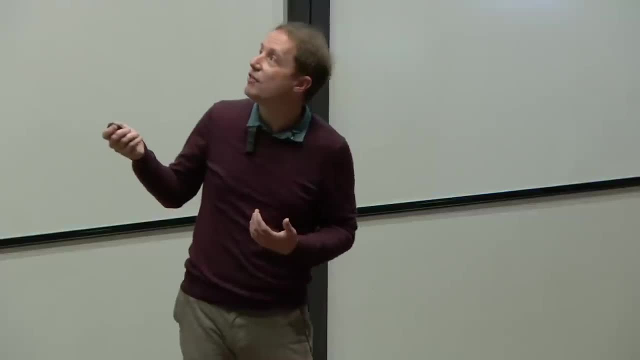 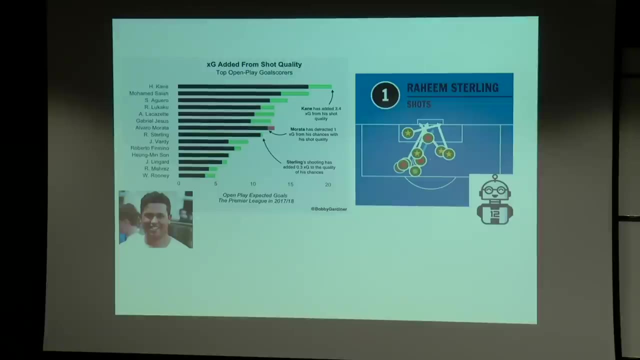 So Raheem Sterling is actually just slightly above average in conversion. So you can actually do that statistical test and show that. And we find actually this season that Raheem Sterling is the top striker, He has the best chances and he's scored quite a lot of them. 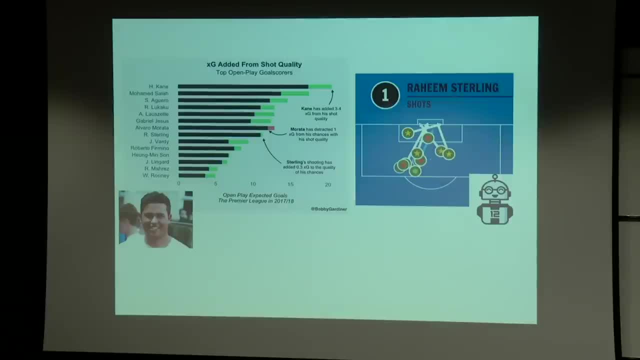 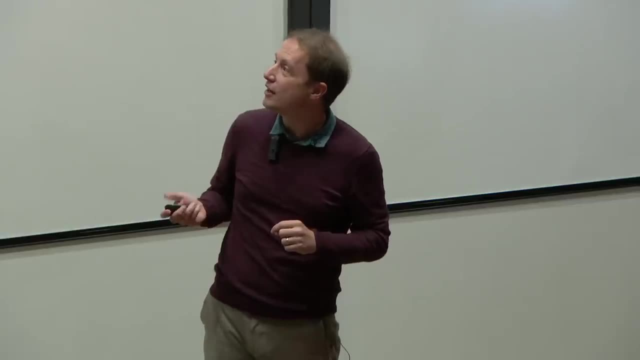 if we do the statistics. But even if you don't believe any of the statistics, I now have the final proof that Raheem Sterling actually is a good striker. I take it back: Vinnie Jones admits he was wrong about Raheem Sterling. 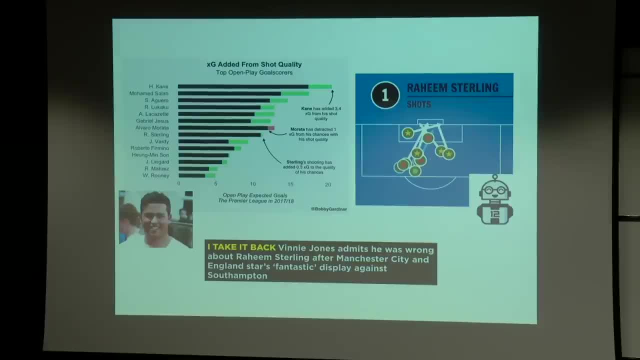 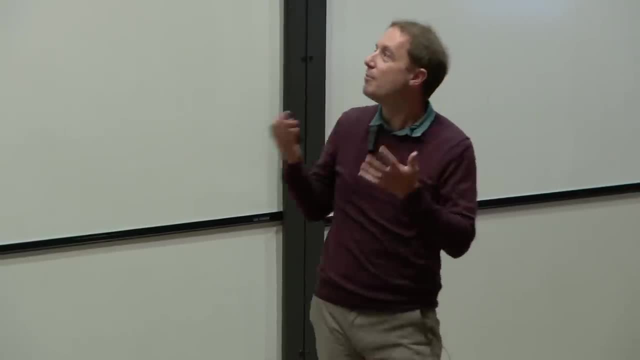 after Manchester City put in a fantastic display against Southampton, And so that's a lot of the time what we're up against, This idea that, yeah, there's this idea that it's all about some sort of passion and it's not just to do. 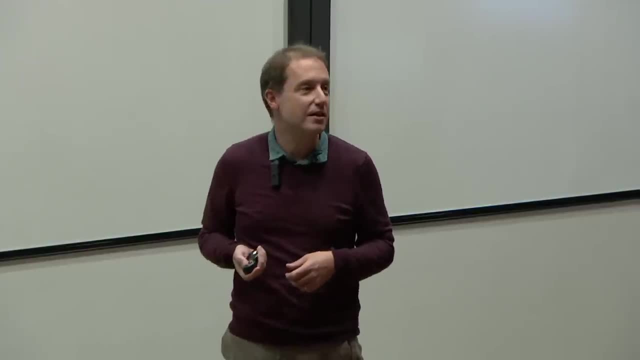 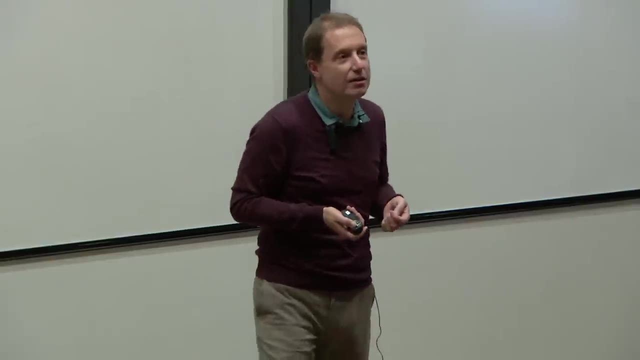 with statistics, But there's often statistics underlying why certain players are the best players, And I would say Raheem Sterling is the best. Statistically. he's the best England player we have just now, And this goes on, So it's another example. 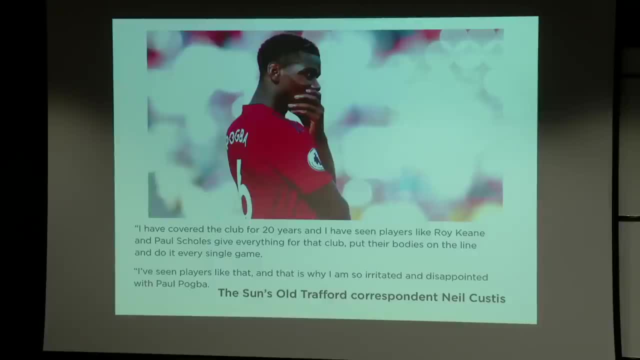 This is Paul Pogba And the Suns Old Trafford correspondent. he said that he basically compared Paul Pogba to Roy Keane and Paul Scholes and said that he wasn't doing his job for the team and he should try harder and do better for Manchester United. 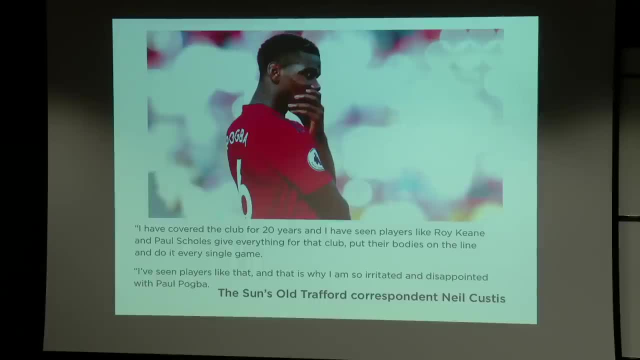 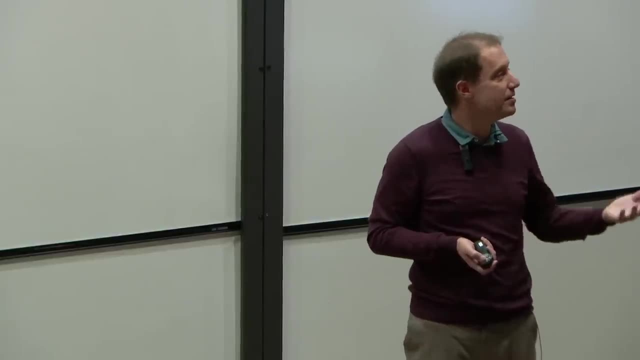 And this type of thing is slightly more difficult to test, because it's easy when it comes to goals. But how do you test a midfield player? Paul Pogba plays deep in midfield. He plays, sometimes assists, but he doesn't always score all of the goals. 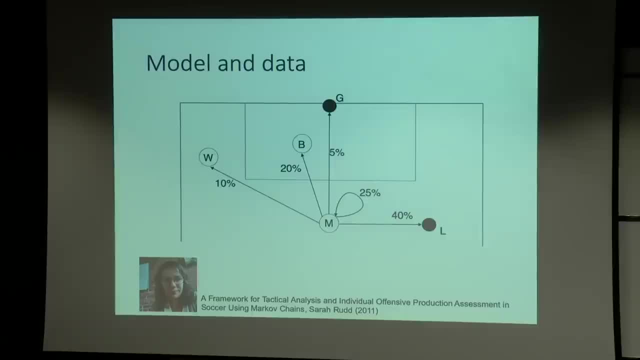 So how do you test this? Well, a solution to this was suggested by Sarah Rudd, who has a- I'm not sure if she's a mathematician, but she has a strong applied mathematics background, And her idea was to use something called a Markov chain. 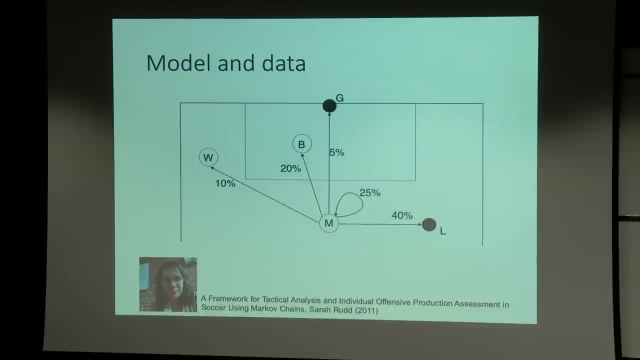 to assess midfielders And the idea is you basically build up a model of the In a typical game of football. what's the percentage chance that a ball in the midfield goes out to the wing? What's the chance that it goes into the box? 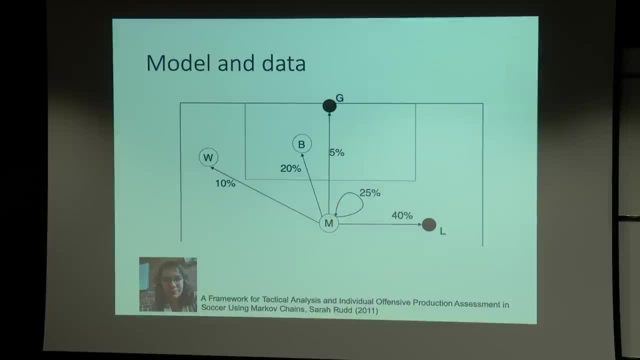 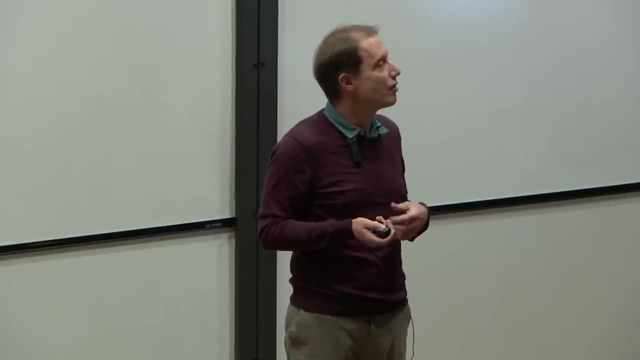 What's the chance that it goes into the goal And you can build up an overall model. assuming that passes in the past don't affect the future, You can build up an overall model of the quality of different types of passes And that framework is something. 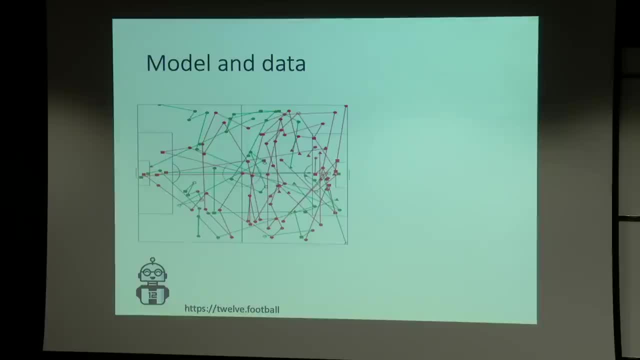 that we've worked with quite a bit and developed. Again, coming back to the idea of model and data, the idea is that we use all of the ball actions in the group and we group them into possession chains, So each one of these, 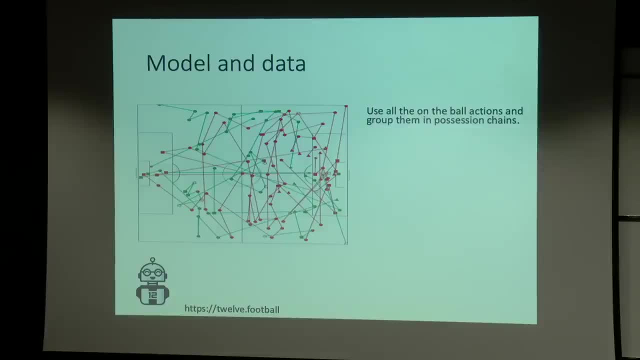 messy lines. here is a possession chain ending in a shot, So it might be a sequence of passes, dribbles. the ball might be lost for a few seconds but then regained, So it's a chain of a possession landing in the shot. Then what we do? 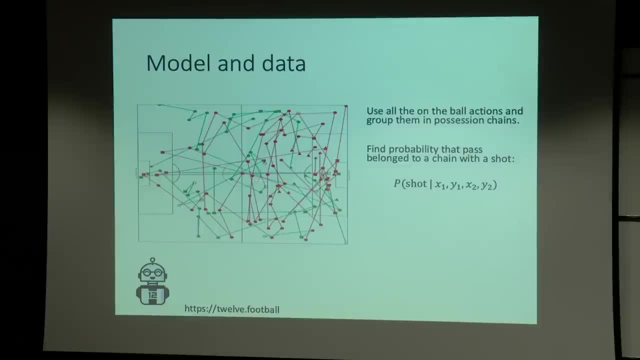 is we find the probability that a certain pass in this chain ended in a shot, And this is really extending the expected goals model over the entire pitch. So we're looking at all the passes. What was the chance that they ended in the shot? 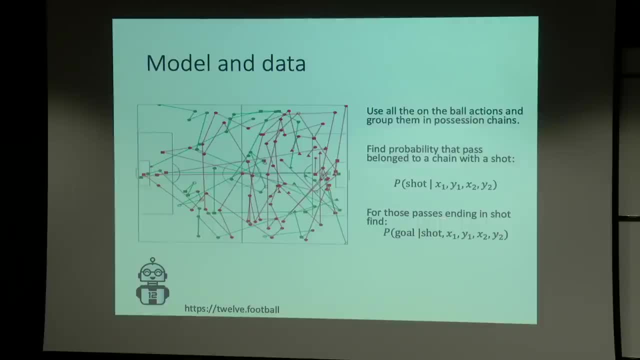 Then we work out- was it a goal? if you have all of these pass coordinates in the shot, And then we do the similar thing, but in reverse, for we do a similar thing for dribbles and then we do the reverse for tackles. So if you prevent, 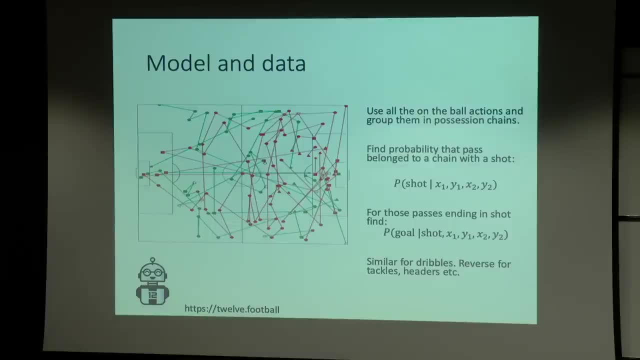 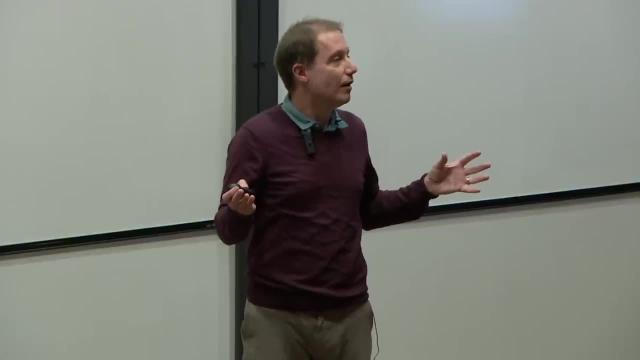 an attempt on goal by the opposition, then you can actually evaluate how dangerous that type of attempt was. And this allows us to build up a model of the whole game of football, assuming that everything is memoryless- that we go from just from one pass. 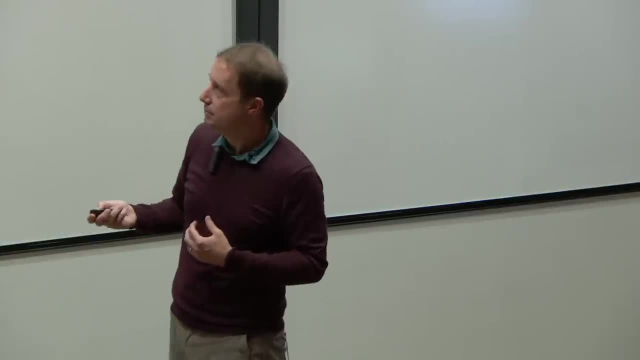 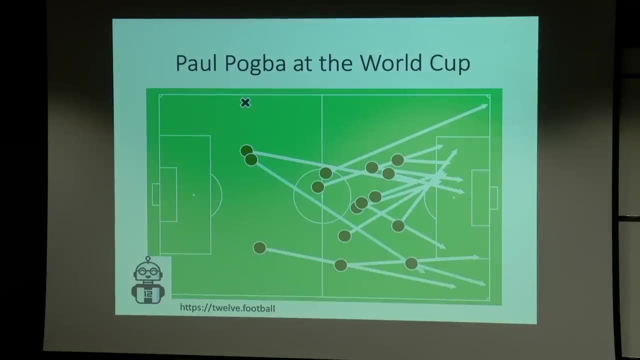 to the other, not remembering the sequence that they were in before And that could then find us. we actually could find that Paul Pogba was one of the most important players at the World Cup. He made a lot of passes from deep here in midfield. 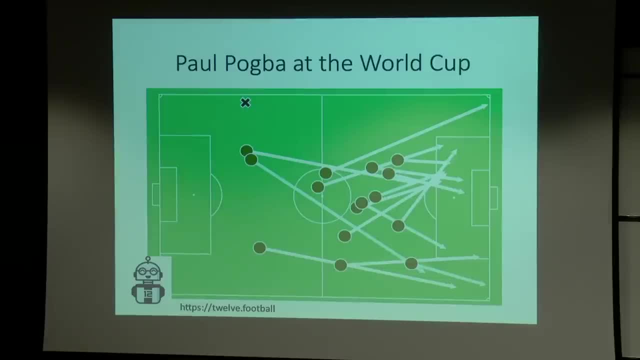 and these are model evaluated as extremely valuable. If you can pass the ball from here to here, then you're going to be able to launch a very quick counter attack, And so he makes a lot of passes that are of extremely high value, And we made a ranking, actually. 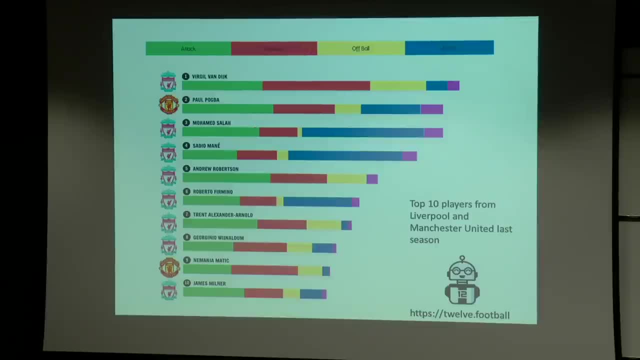 for last season. based on this measure, The green one is the attack value, The red one is defence and the blue one is scoring goals. And I just wanted- I wanted to really rub it into Manchester United fans about who the best players were. 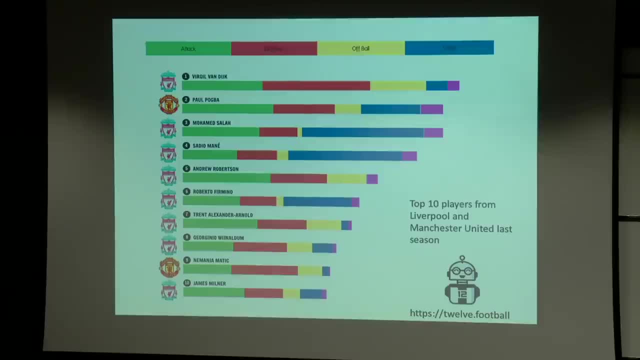 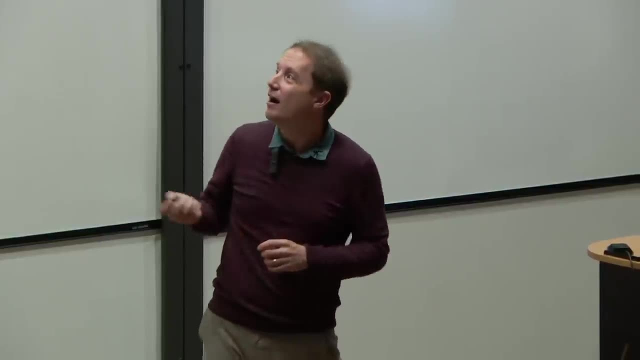 So I use this as an excuse. I just ran Liverpool and Manchester United players last season ranked according to our Markov chain model, And I just wanted to really rub it into Manchester United fans. And it's interesting to see that Virgil van Dijk, 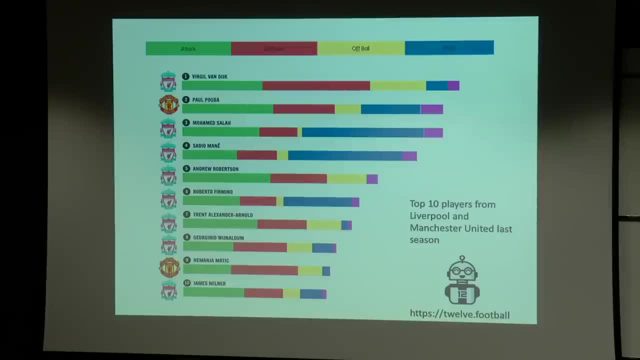 who won European player of the year came out top mainly because of his defensive contributions, But then in second place you have Paul Pogba, and he does everything. He produces lots of effective passes, He defends very well and he has lots. 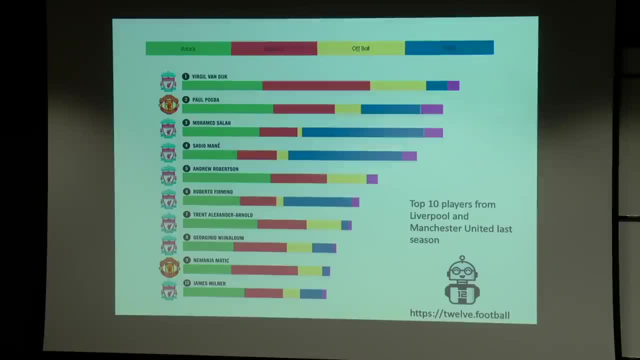 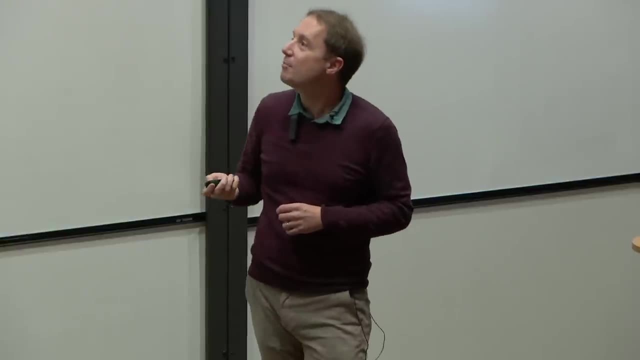 of very good shots and goals. Then you have a whole row of Liverpool players, all the way down to Matic, here, And so we can actually measure the skill of the players, And this is what I like to think of. you know, if you're. 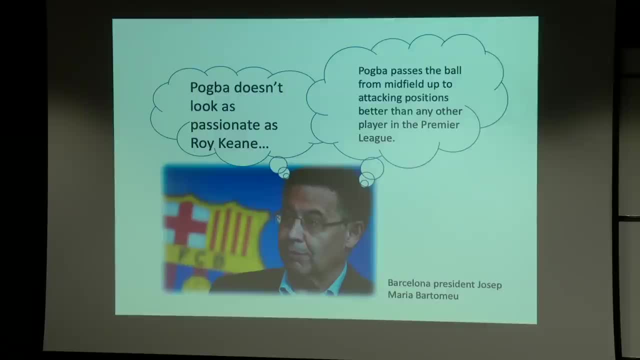 I'm going to come to Barcelona now, where I went to visit. but Barcelona were, for a while, very interested in signing Paul Pogba And I don't think that they think. well, Pogba doesn't have as much passion as Keane does. 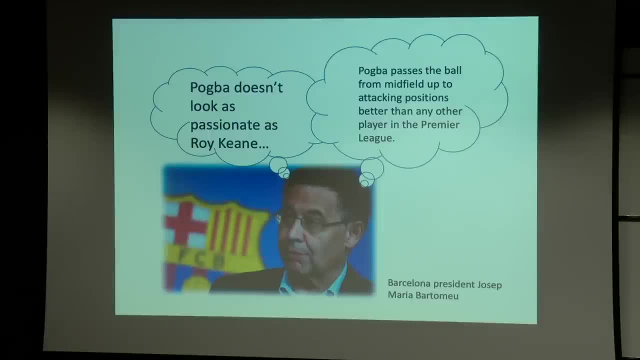 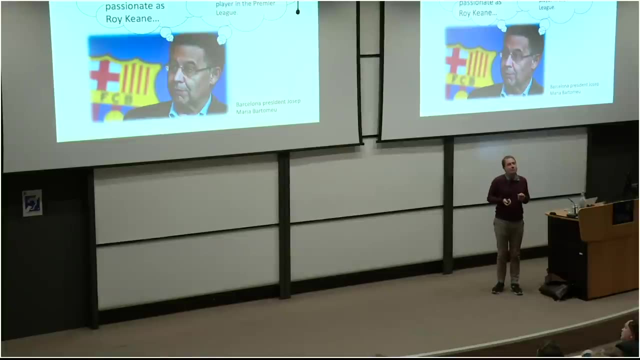 What they're thinking in their mind is: Pogba passes the ball up from midfield in a much more effective way than any other player. So now I'm going to come to my own contribution and how. what I've been doing in football, As I said before, 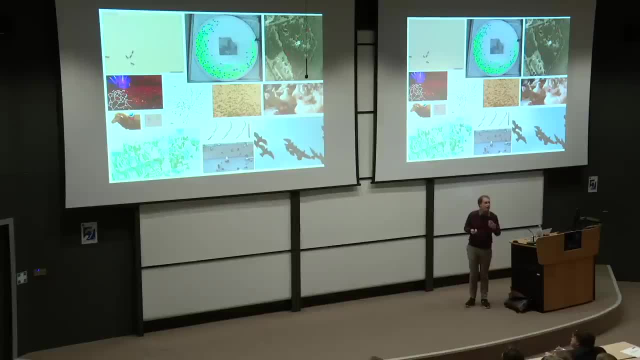 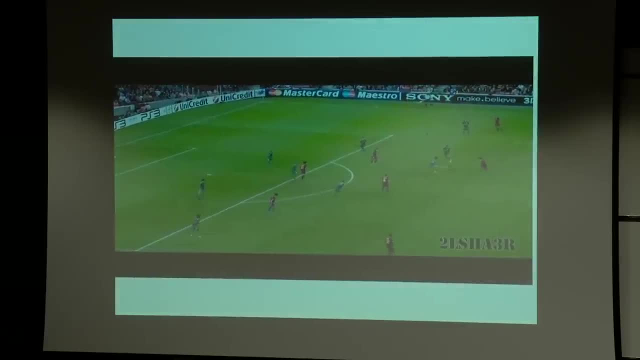 I think we've gone over that. a lot of my work was on collective animal behavior, trying to understand the movements of animals, And then, when I started writing Soccermatics, I became very interested in exactly this type of movement on the pitch. So if you watch Barcelona, 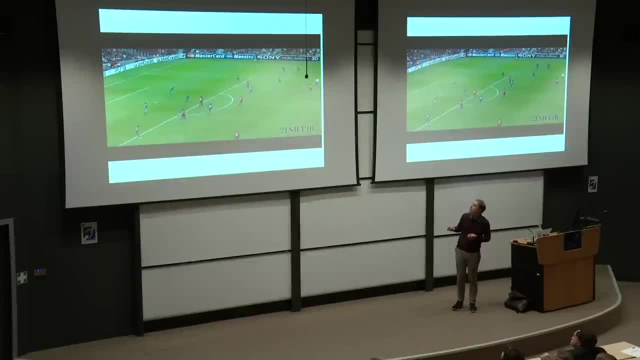 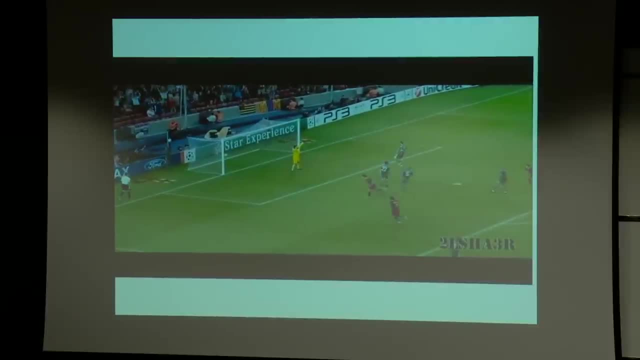 maybe I'll show. this is the Barcelona team of 2010-11.. Lionel Messi: you see him, but what you also see is some very, very nice tiki-taka passes that they did during that time And what we could do. 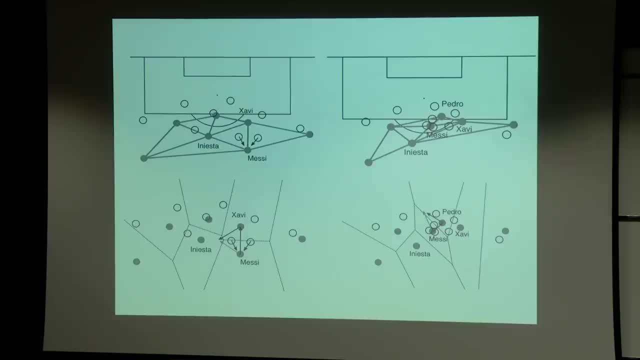 is. we could break down those types of passes by we used something called a Delaunay triangulation, And this is where you connect the nearest neighbors, the most direct neighbors, the neighbors who have a border with each other with a line. 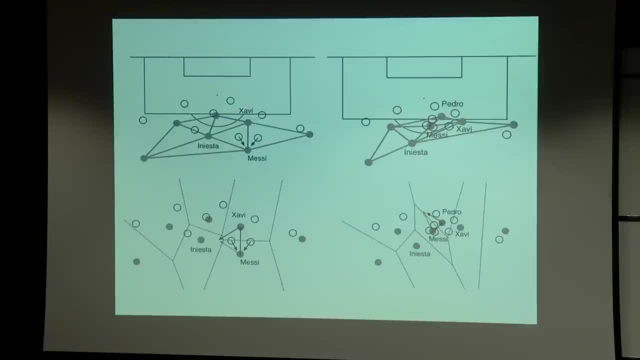 and that gives you a triangulation, And what you see is that Messi opens up a lot of passing. to Xavi, for example, He has an open pass to Iniesta. he has one hair out to the right And if they do this, 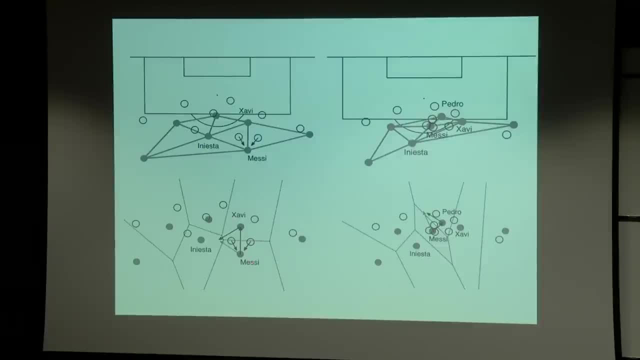 if they stand in this way, where they're kind of maximally distant from other players around them, this Delaunay triangulation opens up automatically, And so this is called a Voronoi diagram, And it turns out that a lot of what Barcelona do. 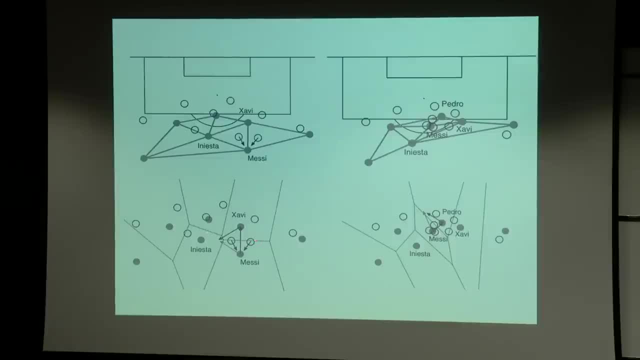 is that they stand in a way which puts their opposition on the edges of the Voronoi diagram, which means that they're maximally distant from them at any given point And, as a result, this triangulation opens up where they can actually pass. 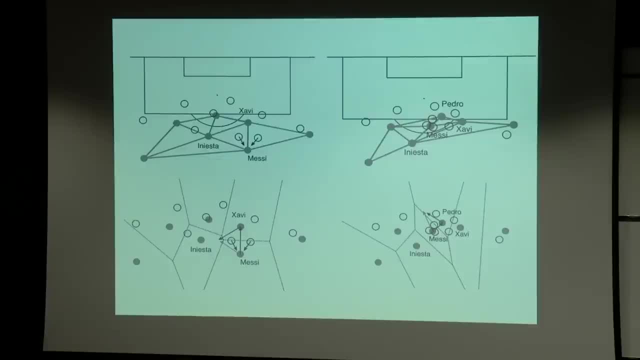 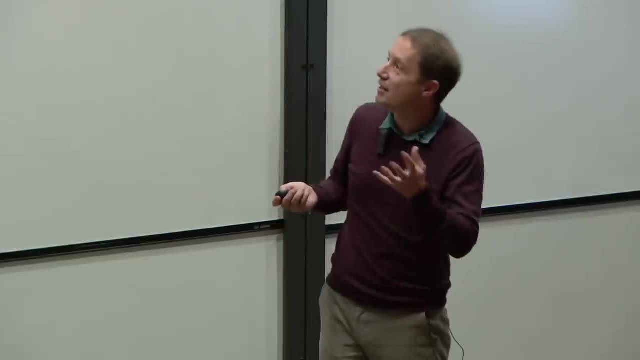 the ball very effectively to each other. So there's a kind of mathematical principle underlying the tiki-taka football that Barcelona have been playing, And I was very excited about this and I wrote a lot about it in Soccermatics, And then I was lucky enough. 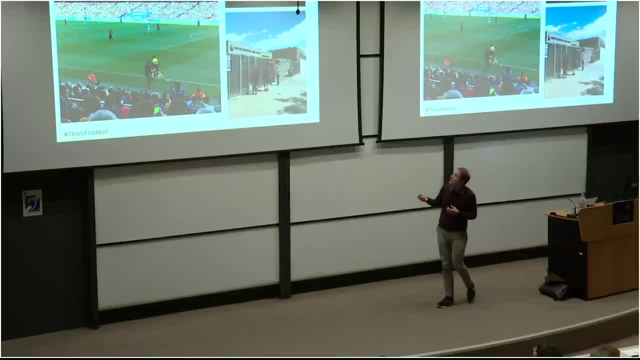 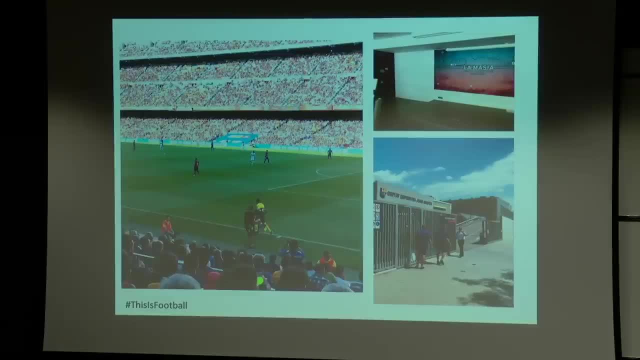 to be invited down to Barcelona and see this is Messi up close and personal. So I got to see Messi really near in action. I didn't get to meet him, unfortunately. I was probably at one point I was at this training ground. 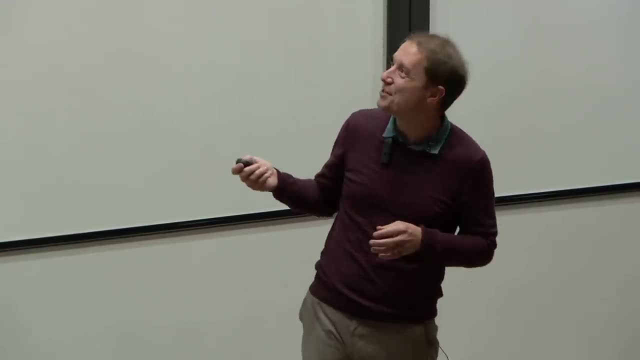 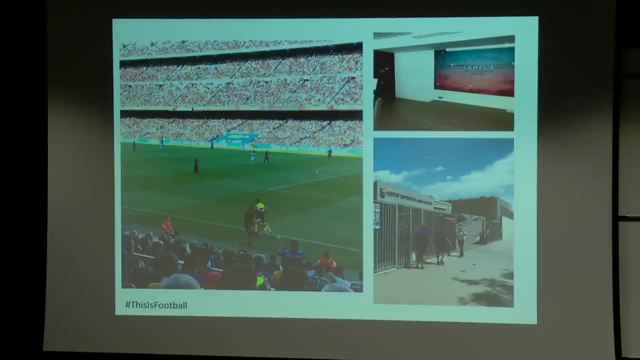 so I was probably a few hundred metres away from Messi when he was training, and a hundred metres away, but I didn't get the introduction, unfortunately. But I did get to meet the data scientists who work at Barcelona and they actually have a team. 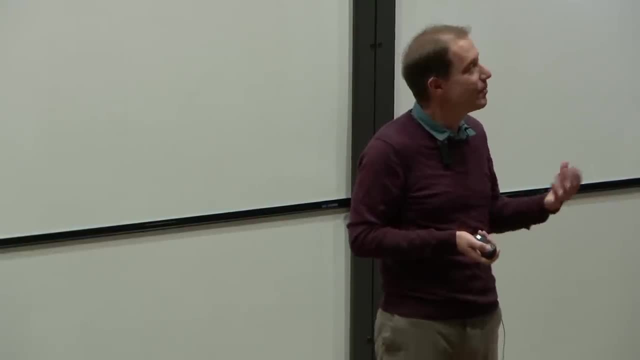 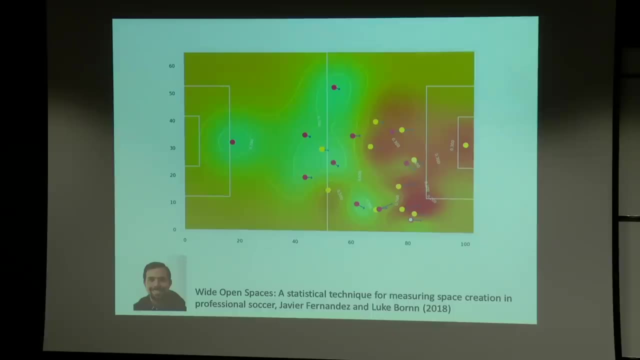 It's a little bit like a sort of university department there, with all the sports science they do. It's a really impressive place to see what they're trying to do. And I met this guy here. This is Javier Fernandez, And I was, of course. 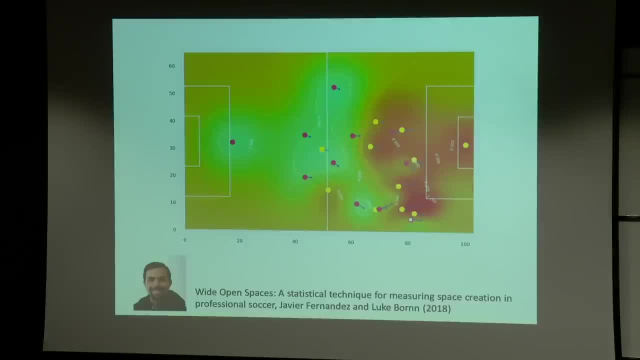 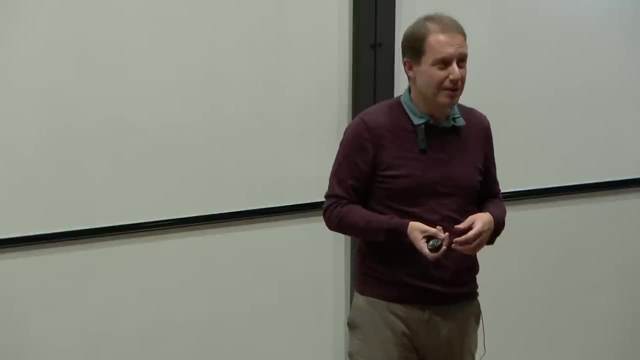 very pleased with all my Delaunay triangulations and Voronoi diagrams And I gave a presentation there and told them all about it And they were like, yeah, yeah, of course we know all of that And I was very surprised to hear. 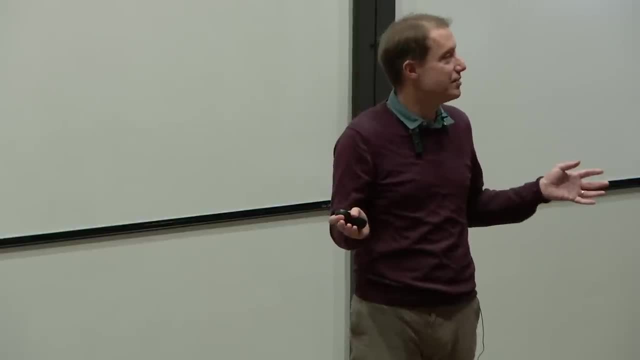 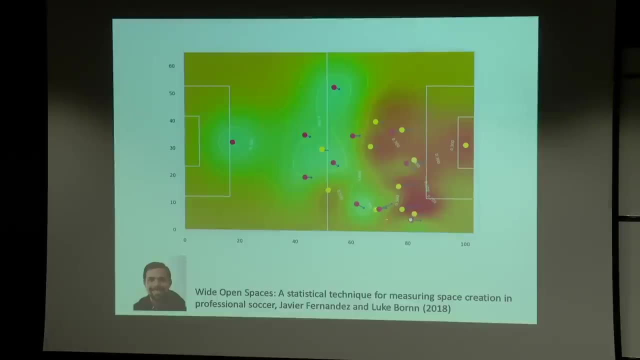 that they already used that type of technique, And what Javier had developed was an even better technique for measuring, basically who's going to come to the ball first. So here is Barcelona playing in purple, and the green areas show where a Barcelona player will come to first. 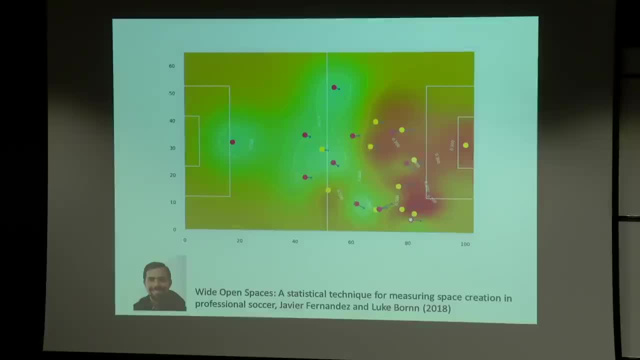 The red area show where the opposition players will come to first, And this they track for every match and they're able to see how the team controls space. And the whole of Barcelona's game is built up about how you can control space. And Javier is sitting there. 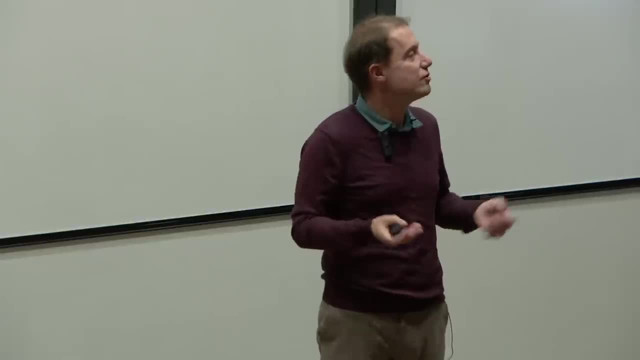 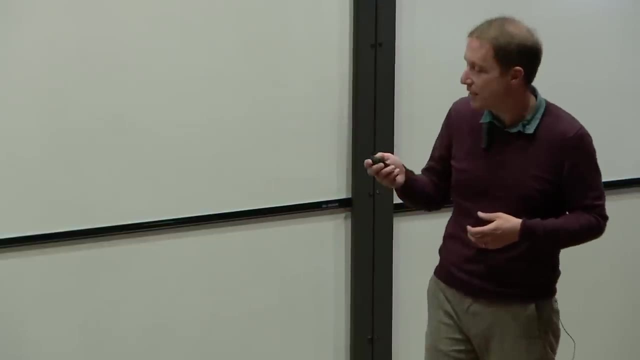 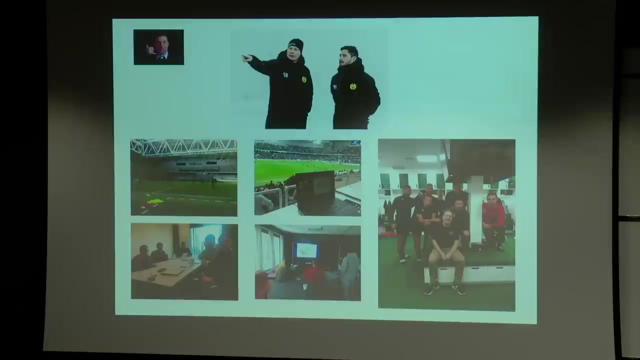 after the match looking well, have they controlled space in the way that they said they would control space? And he can actually give feedback and so on about how they're controlling space. And so I took a lot of what I learned at Barcelona and now I have a research project. 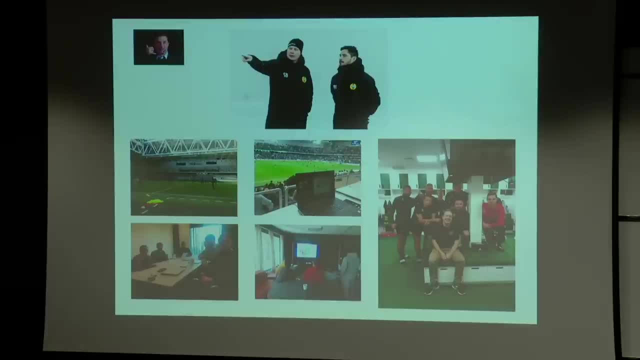 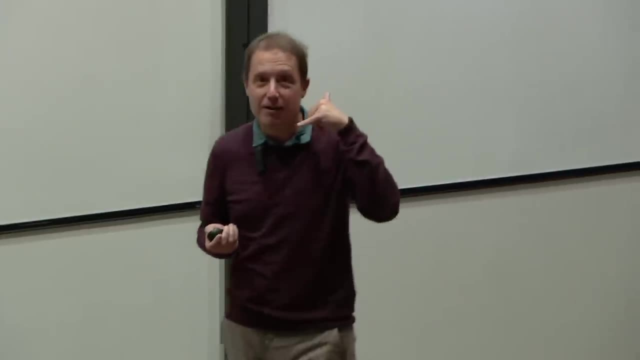 together with them and wanted to put that into work in Hammarby. As I said, this started with me phoning- virtually phoning- Jurgen. By the way, Jurgen, you know you can actually still come and contact me. 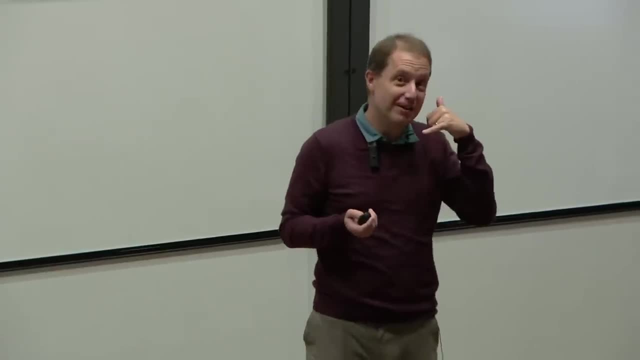 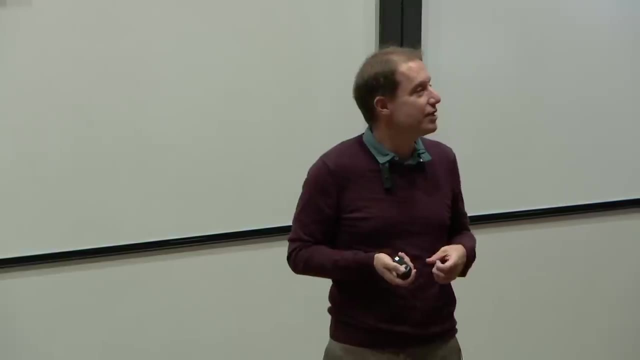 I am a Liverpool fan, so I would rather be working for you. So yeah, But so this started with me making this, and Hammarby did ring me up, and they're a local team in Stockholm, So it was much more easy for me to start working with them. 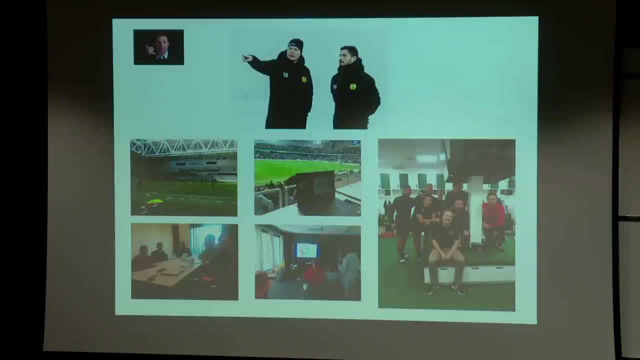 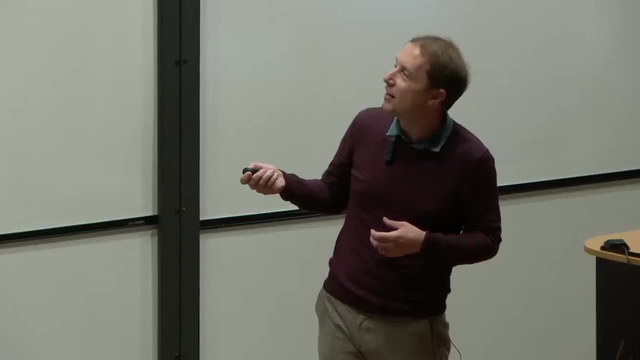 And their coach, Stefan Bilborn. he was very open to this type of this type of collaboration And now I often go to the trainings. We have development things here And what's most fun is that we have a feedback cycle where we can present. 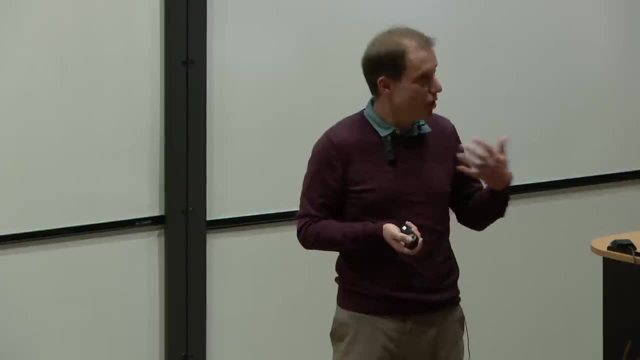 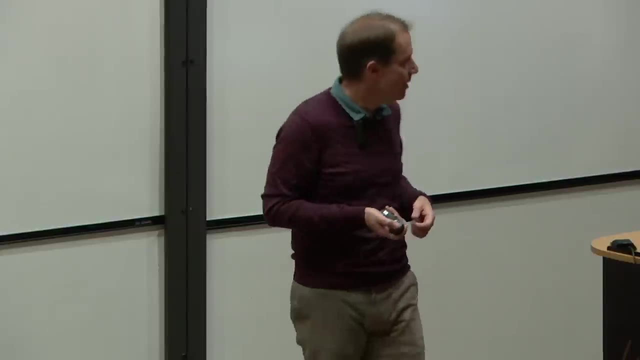 what we've learned to the players and show them mathematical models, And they say whether they think that this works or we can actually give them feedback on their performance. I'm going to give a few examples of this. One is exactly as I said. 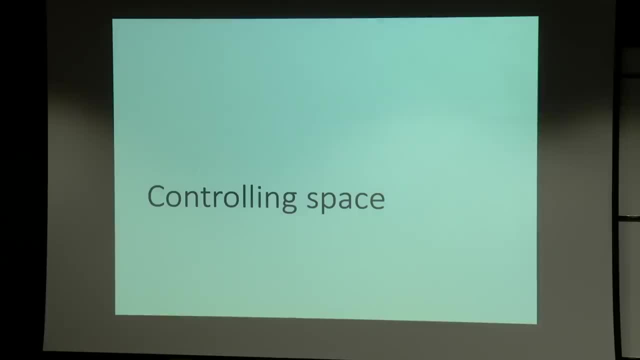 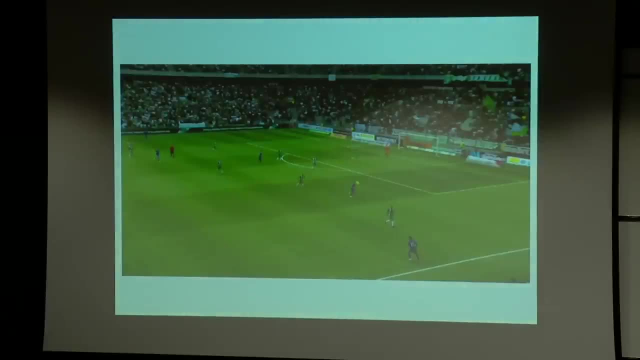 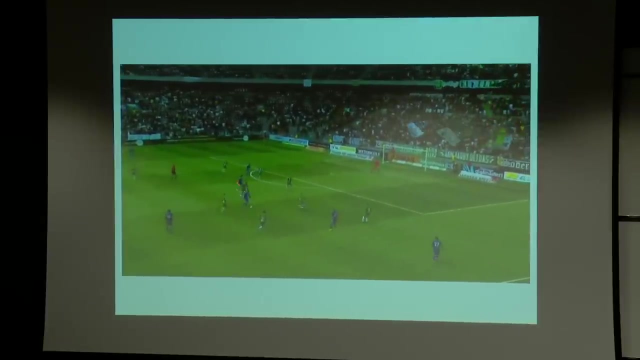 this was Javier's method that he's been developing. We've been developing along that idea. This is a goal that we scored recently. We're the green team here, So you're cheering for the green team now, right, Okay, so if the blue team score, it's bad. 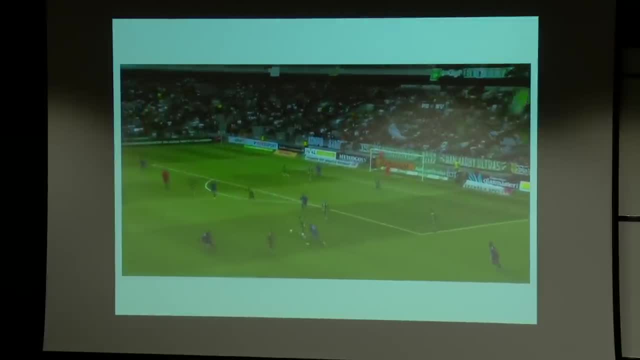 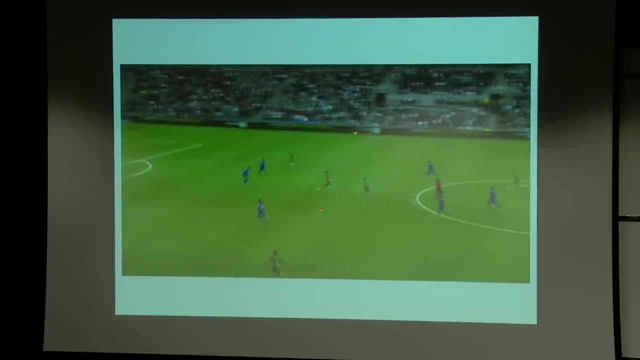 Green team need to score, So, oh good, We've got the ball back. This is Mojo Tankovic, who's our best-ranked player just now, according to our system. Alex Kachinichich, who played for Fulham. 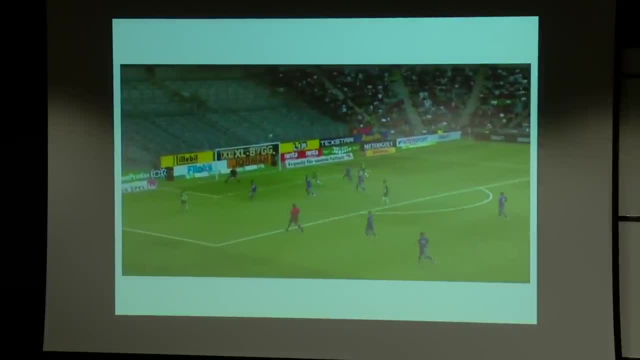 Both of them played for Fulham. at one point Get the ball out to Niko. Niko gets it back into the middle And Mojo, who got the ball back in the first place. he manages to score a goal And he's very happy. 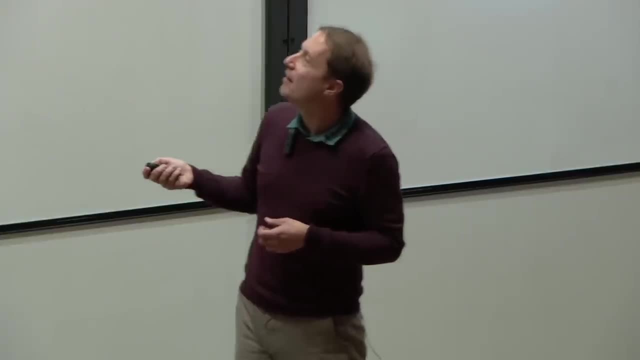 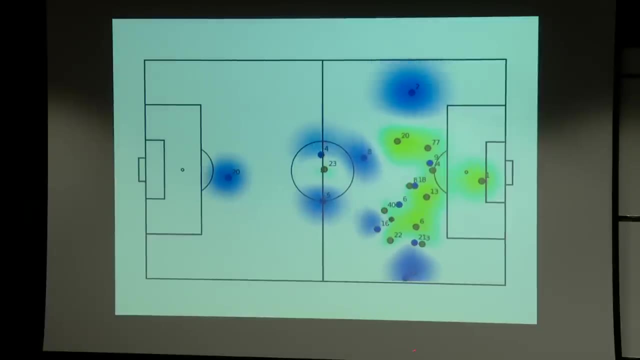 And what I like about this goal in particular. and now we're going to do the same thing, but analyse it from this top-down view, And I'll just let it play to start with so you can get a feeling for it. So this is the opposition. 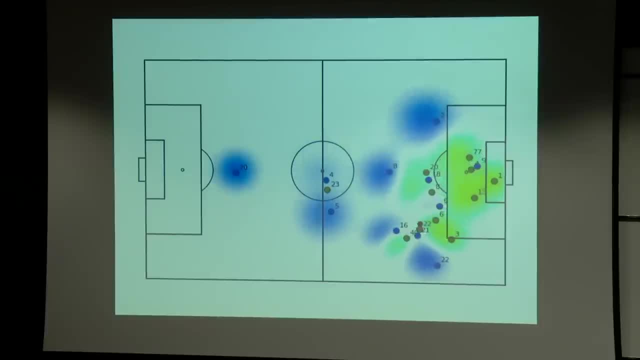 It's Sundsvall attacking. They take the shot. The ball comes back. Mojo is 22.. He collects it. Niko opens up space here. Alex opens up space here. Niko's still got this lovely space here the whole time. 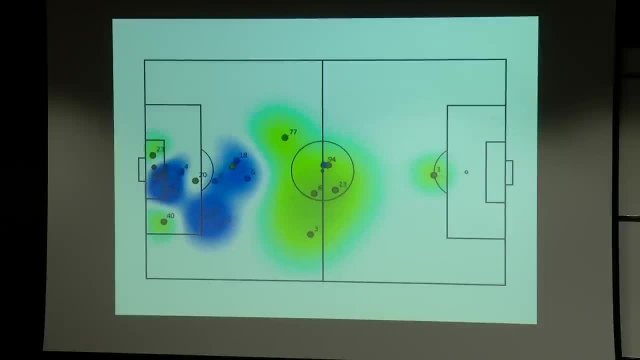 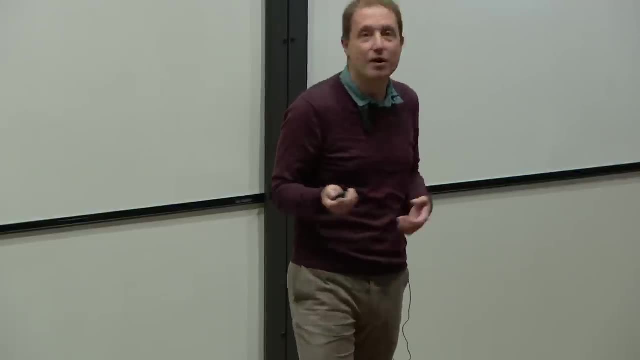 Keeps it, keeps it, keeps it. Then the attacking players come in and score a goal, And so we can actually see how they're controlling and using space in the build-up for those goals. These points are very important because one thing we talked about a lot: 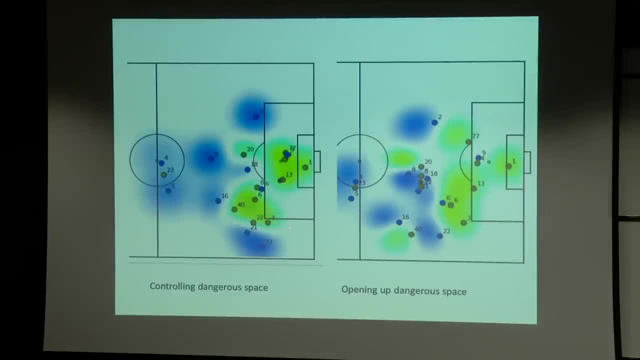 was defence. You need to come back and defend, even as an attacking midfielder. Mojo is a player who always wants to run up and score goals, But if he's standing around here, then we actually. when the shot comes in and it's controlled by the defender, 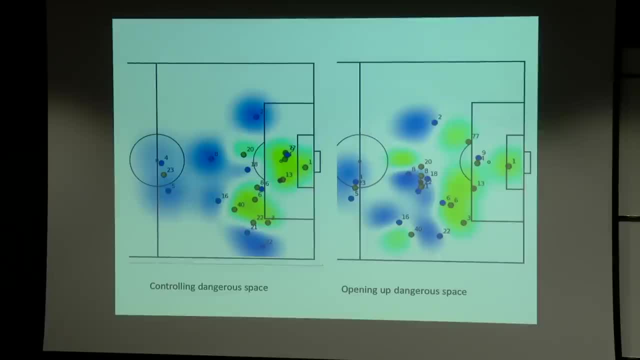 or it's headed away by the defender. we control a lot of the area outside our box and they don't control it, And so, if you think of the ball as just sort of bouncing out at a random direction, we're going to control a lot of the places. 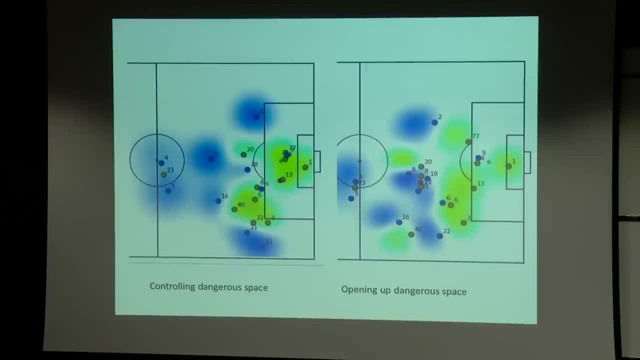 where it could bounce out to. And here's another where, a few seconds later, you see Alex controls this space in front of him. Alex is number 20.. He's running in this direction. Niko is number 40, running in this direction. 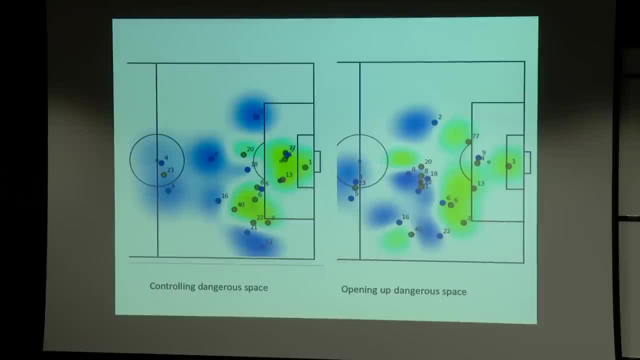 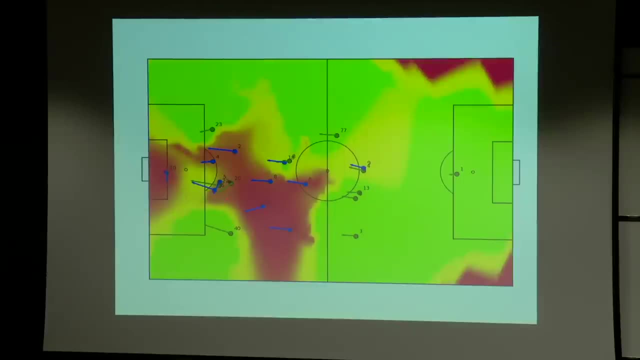 And they've started to control the attacking space on their way out, And so you can actually get an idea about what spaces we're controlling. Another thing you can do is you can look at pass probabilities. This is when Alex sent the pass out to Niko. 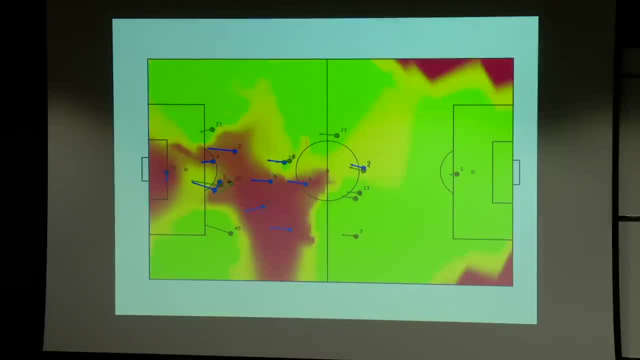 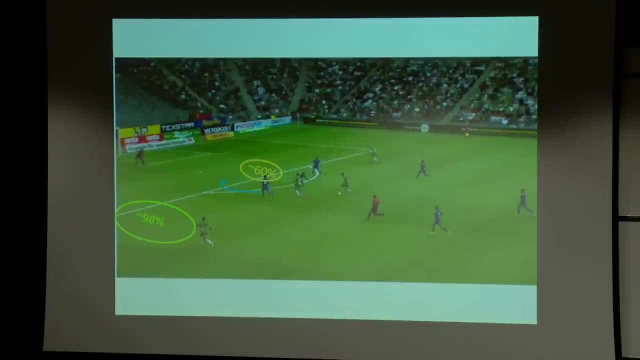 This is basically 100% success rate expected from our model. We calculate all the possible passes he could make And we could say Alex could have tried to play the ball through to Mojo straight away. We have a 60% on that. 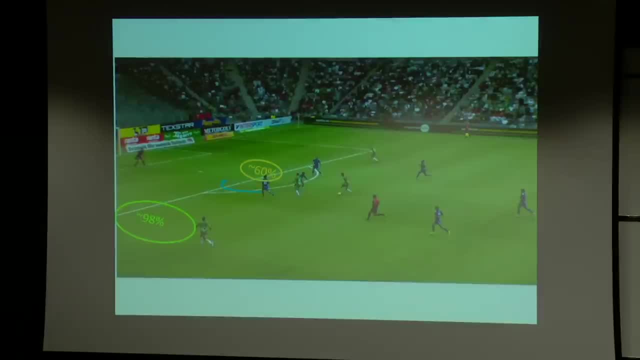 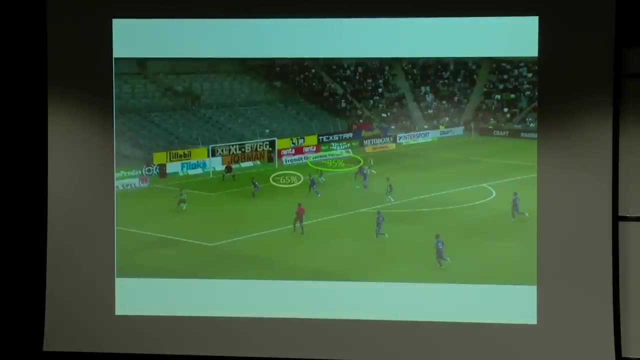 But he has a 98% chance if he passes through to Niko. Then a few seconds later we have this situation, And there we found out that now Niko has a 65% chance to Mojo. He could have also taken the post further away. 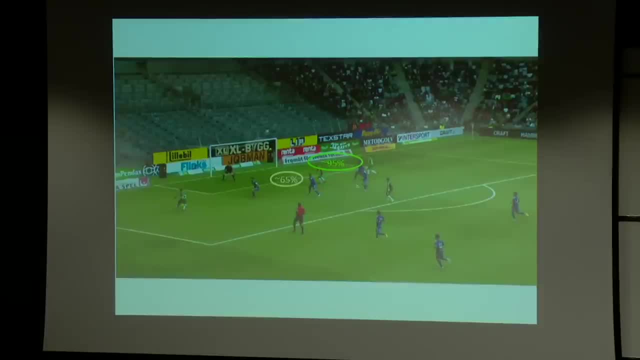 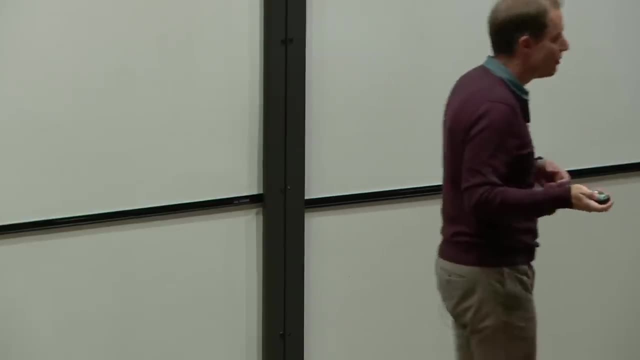 But if he takes the post further away then he's got a worse angle for the striker there. So the best decision is to take the 65% chance which he takes and they score, And so we can use this type of technique basically to improve the position. 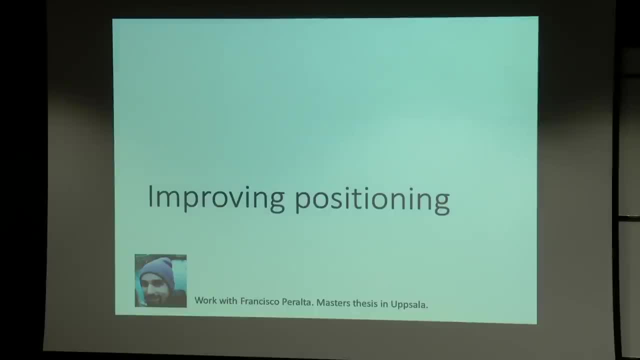 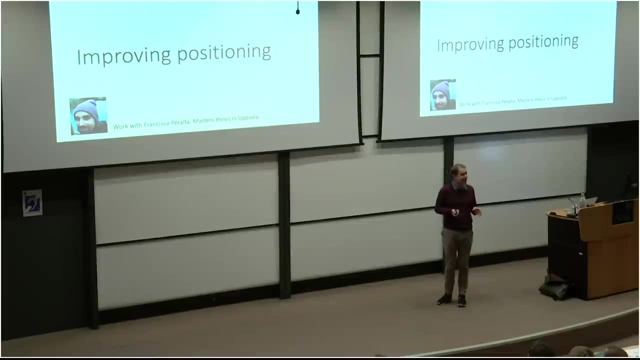 This is a project together with Fran Peralta, who did this as a master's thesis. I've become incredibly popular in my university when it comes to writing master's thesis Like. I get a lot of requests to do this And most of them do. 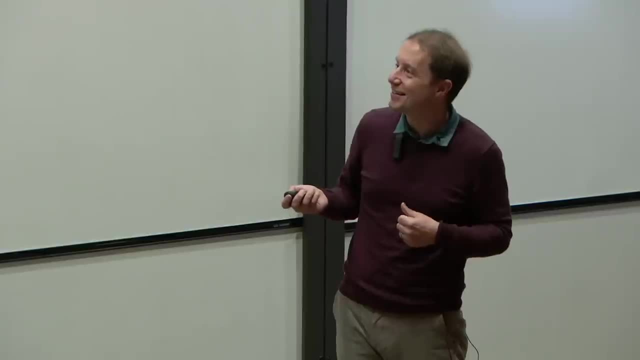 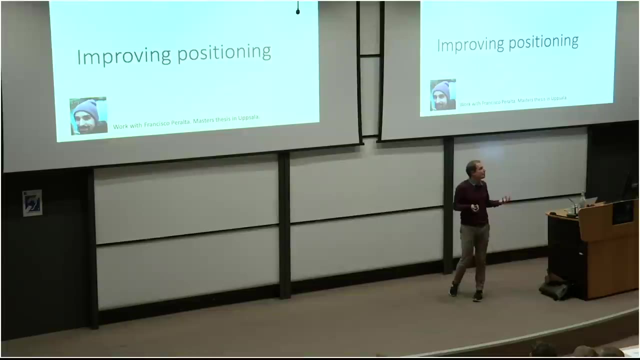 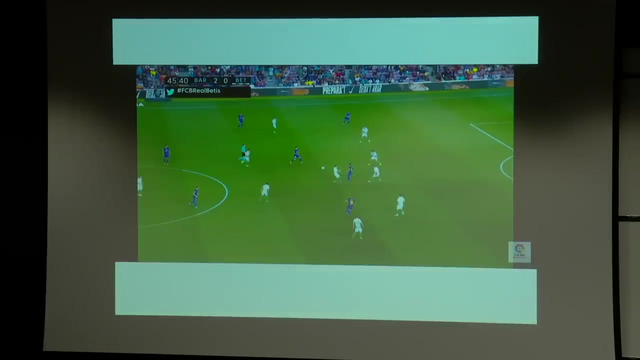 I do manage to find time for them because there's so many exciting projects to do in maths and football. But Fran wrote a master's thesis doing this And what our idea was. we can actually feed back and improve the performance of play, And I thought I'd take another example from Barcelona. 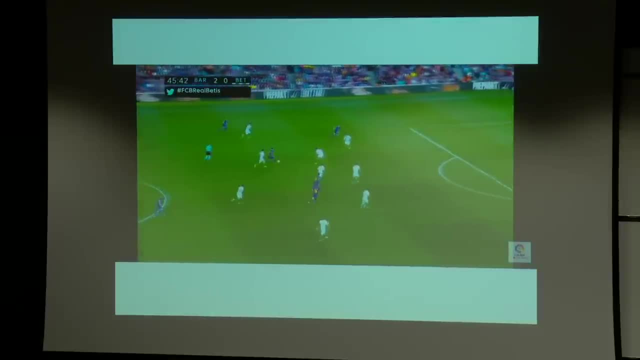 I think this is a lovely. So what do you think is the most important? Maybe I'll have. This is a sort of test. What's the most important thing that happens in this sequence? Have I got any suggestions? Anyone? Guy on the left is very important. 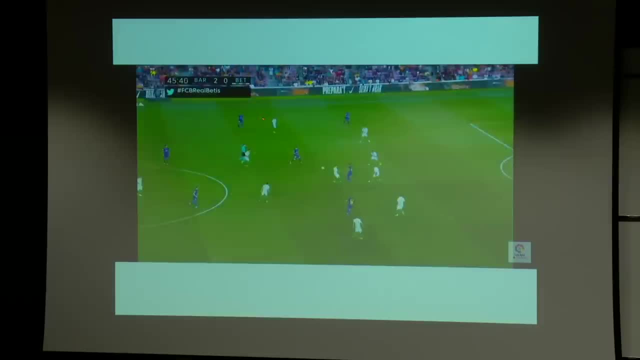 He runs and gets the ball. Is this the one? you mean The guy who runs past the goal and runs far left Him here? yes, He gets the ball, so he's very important, But I think that the absolute most important thing. 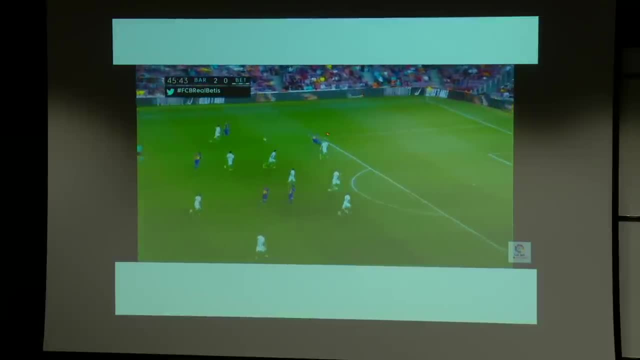 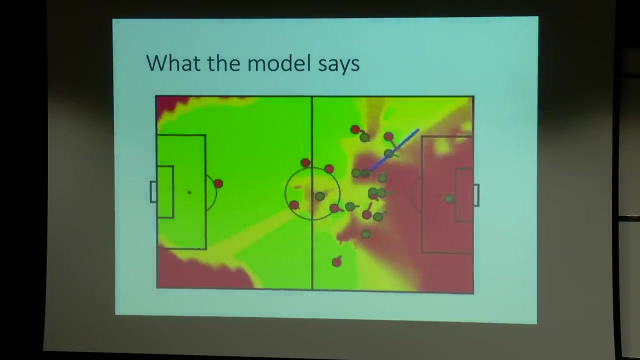 is this run here? Because what that run does is it opens up space for the player on the left so he can run through onto it, And you can actually see that in this picture. So here is the top-down view. again, The ball is coming from here. 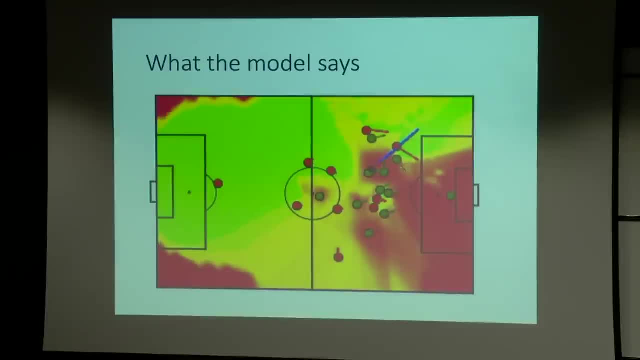 and the pass is going to there And you can see as the player, As the player here, moves inwards, it opens up a green space for Alba on the left, And so it's the movement actually opens up for the other players. 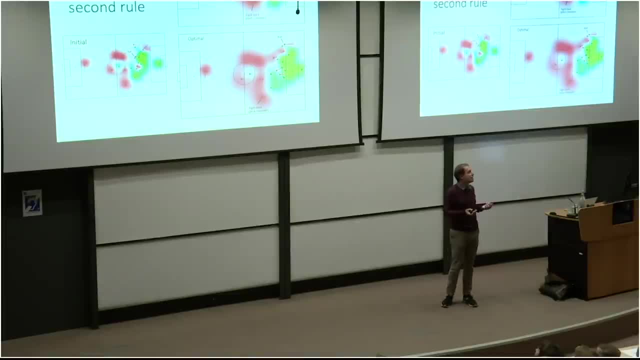 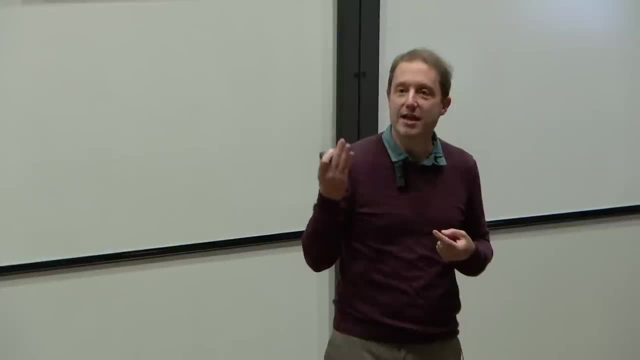 And we can actually simulate how the football players move, And this idea comes from a lot of what we worked on with animal behaviour. We can simulate one or two seconds into the future, Because when animals try and avoid colliding with each other, they tend to anticipate. 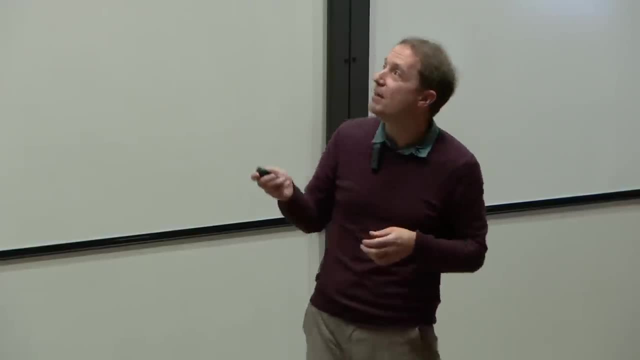 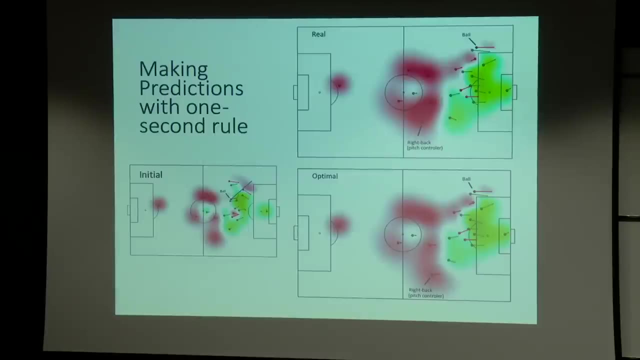 where other animals are moving to and move into open space And so we can anticipate what happens into the future. We can say to the players: you can anticipate what's going to happen into the future. Where should you move optimally in such situations? 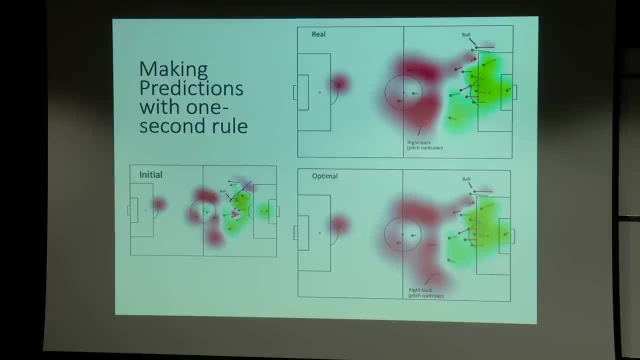 And we can simulate that This is an example of a right-back. He was quite a long way from the play. We have an optimal position. he should move out here. In fact he moves quite centrally, So he doesn't really move in an optimal position. 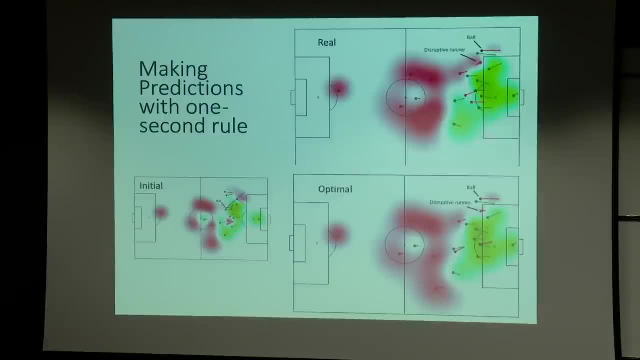 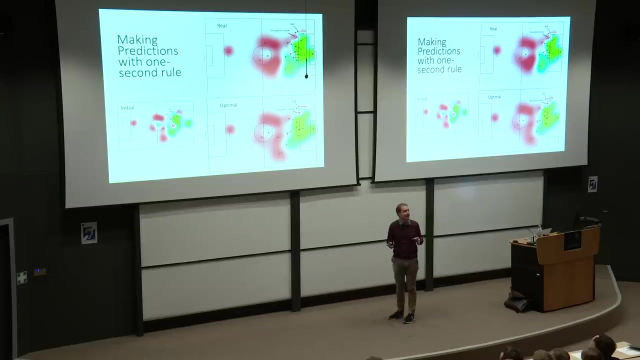 But what we actually find about the attacking midfielder here is he did move in a perfectly optimal way. So his run- If you look at the run, he runs like this and then he stops like that, And you could classify that as being quite lazy. 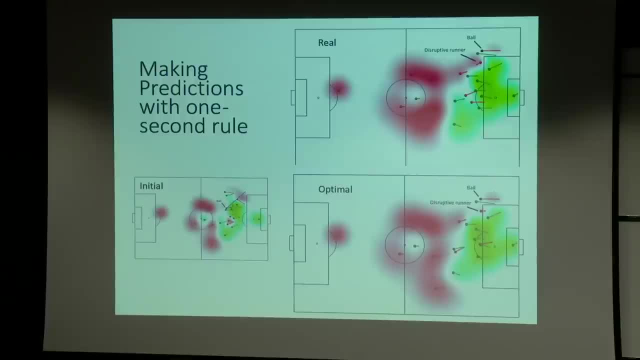 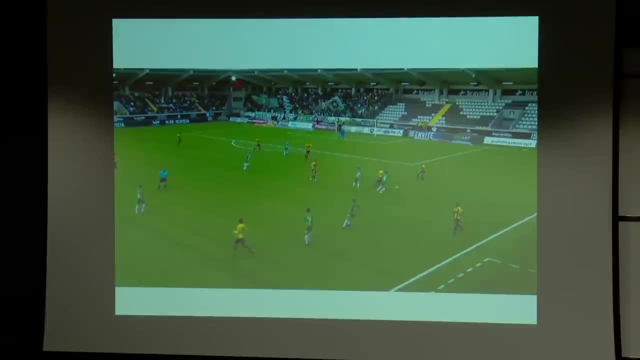 But the way he stops when we calculated in the model was optimal. He had the best stopping position And this is the sort of thing that we can use with the players And we've been doing this at Hammerby. We're basically starting doing this. 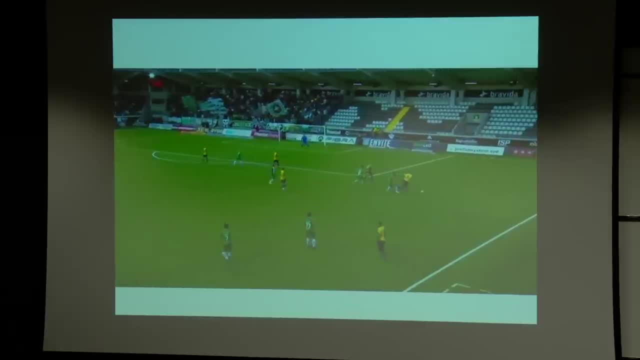 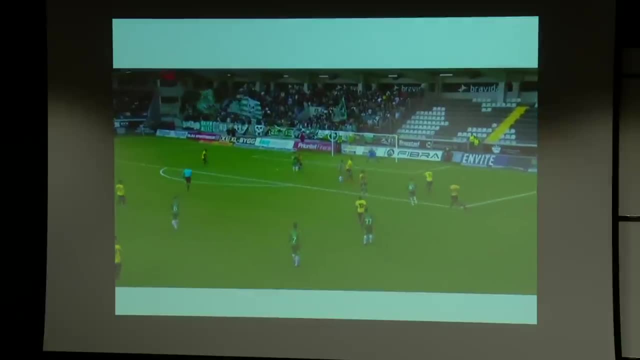 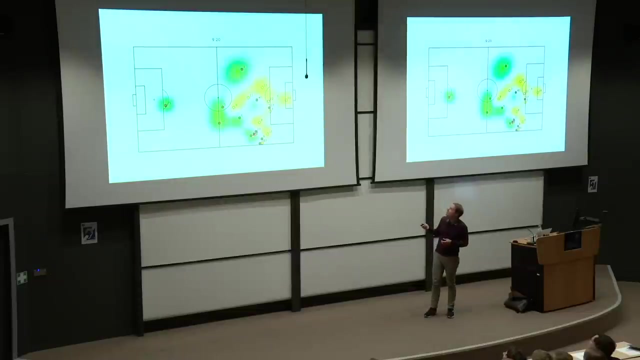 at Hammerby just now, Where we can give them feedback. So this was a very nice example where we got the ball back. He shouldn't shoot from there, actually, So we'll forget about the shot. We talked about that too. What I'd like to point out here: 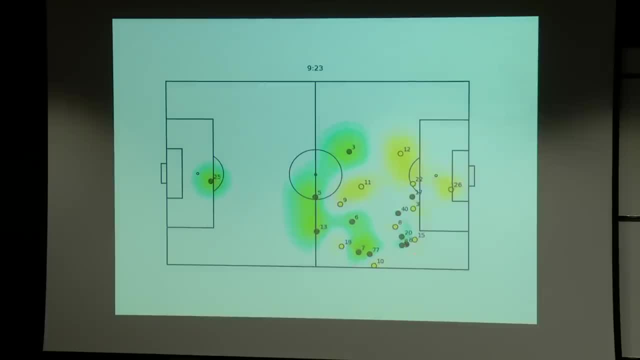 is that the press play here. So they've got the ball And we organise. so we've got man marking very nearby. But we also control all of the space So we can measure how we're managing to press them and how we're controlling. 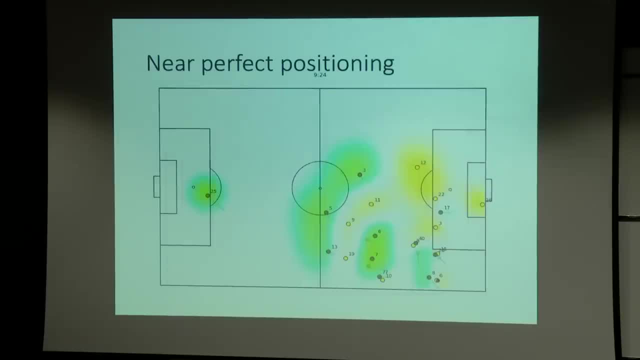 the space around the team And we could calculate with the. This was their actual position, is the shadow picture, the shadow dot and their real position? And we could actually see the players afterwards that you were pretty much optimally positioned in that type of press. 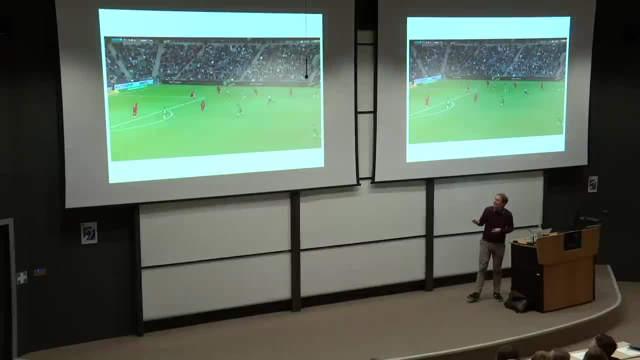 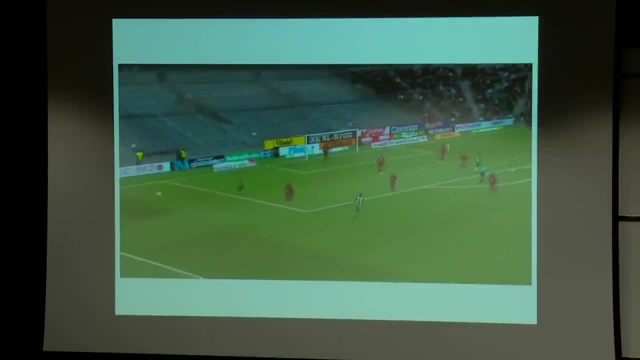 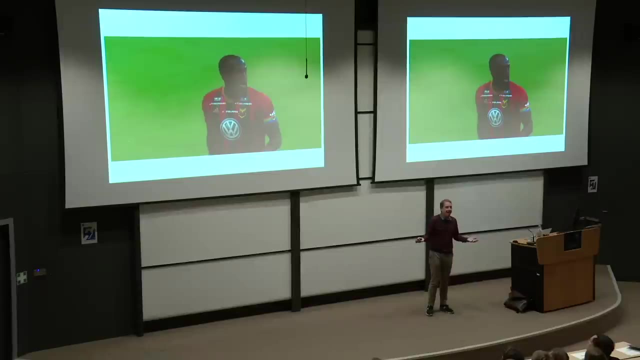 I'll take the question afterwards. There's lots we can do. This was one of my favourites because- Can I say another thing about football players? They're so sweet Like you see them out on the pitch and they're like really angry. 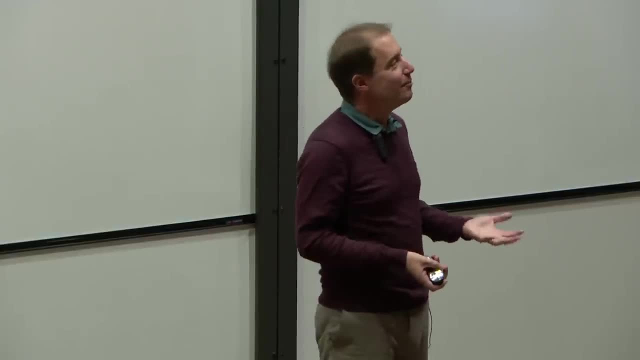 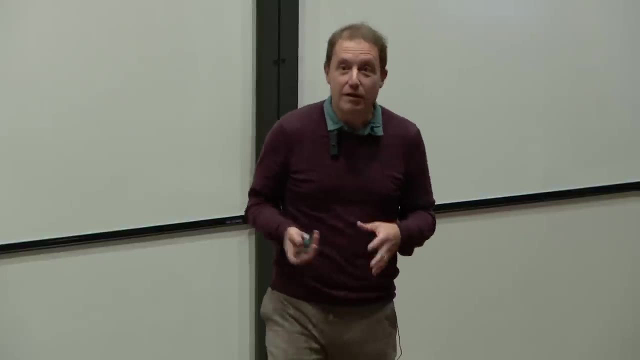 Should have been a foul referee, But like, when you meet them, they're like the nicest people you'll ever meet. They're really sweet And mild mannered And, David, you know it's okay if you tell me about this or something. 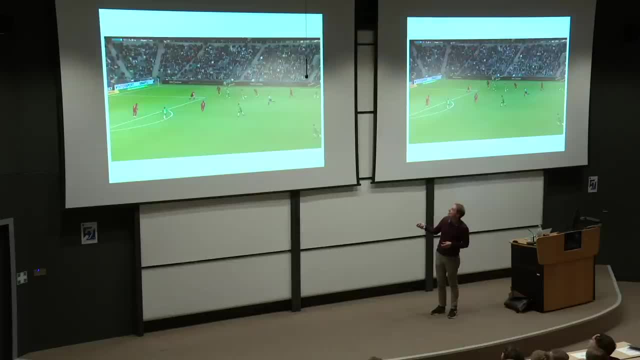 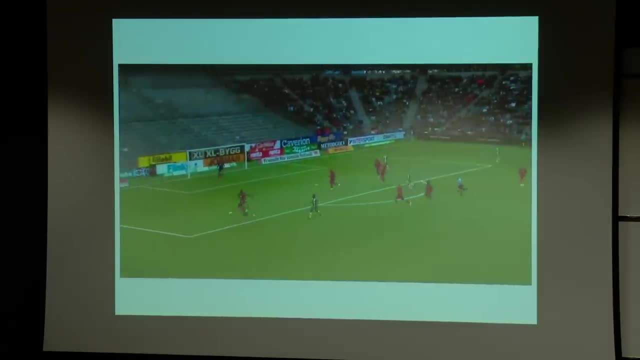 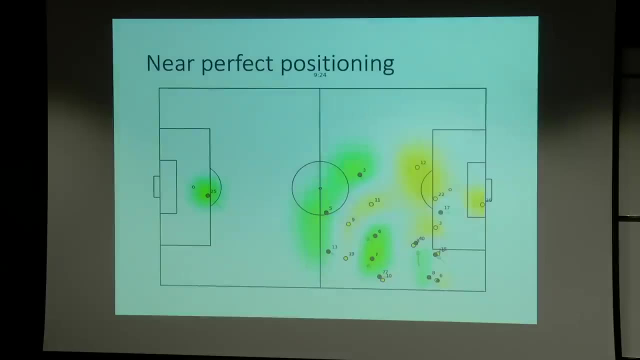 And this is an example. So this what I was just showing here, this is Emad Khalili. He played the following pass And it went out there and it didn't get to the player And, if you, I want to show this one more time. 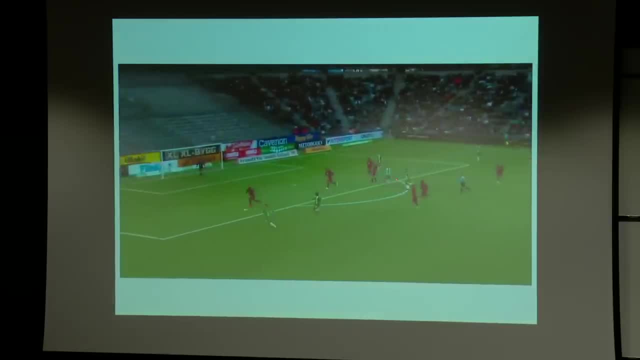 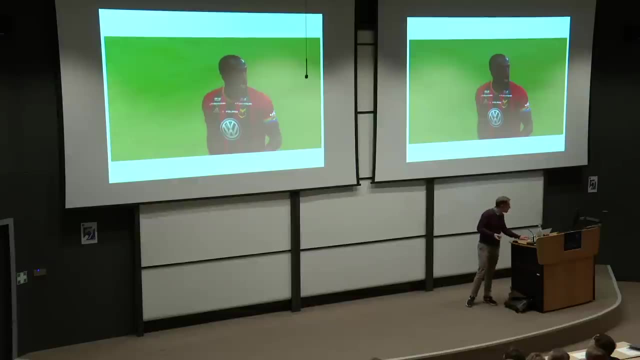 Here we go. If you look at Moyo there, he's like really annoyed With Emad Because he wanted the ball and Emad didn't pass into it. And so afterwards Emad asked me: you know, did I make the right decision? 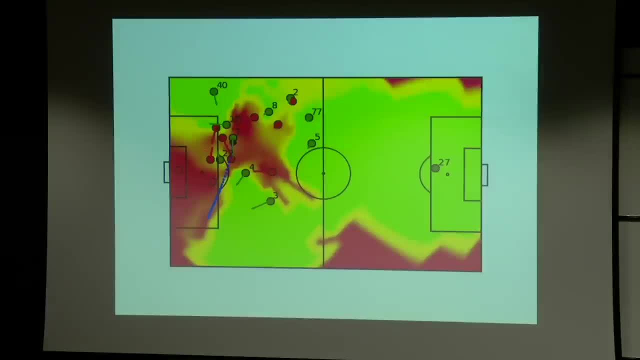 in making this pass And you could actually see that, given the percentages, there was a very small margin that he could get it to Moyo And though the ball didn't quite get to the left back, it was the right decision to play that pass. 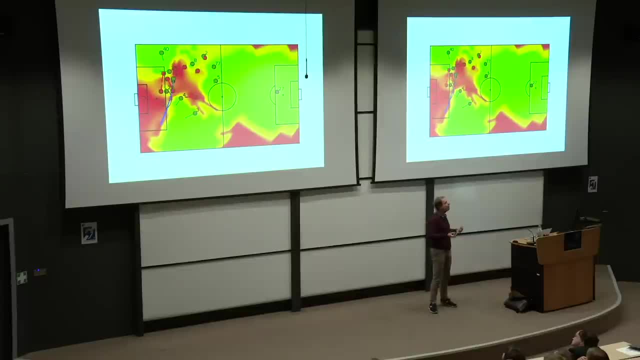 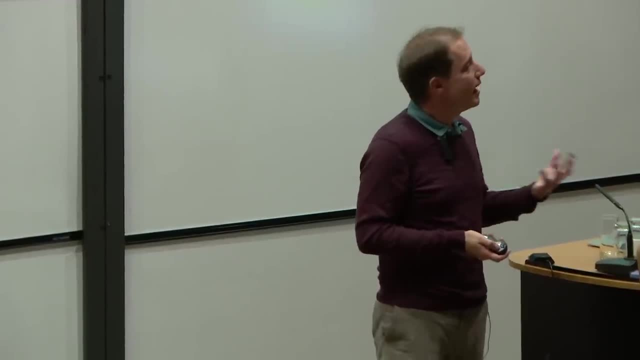 So you can actually use the model to evaluate how you're playing after the game. Right, That's a lot of my experience and how it's been working out in using this type of mathematics, this type of applied mathematics. And now I come back. 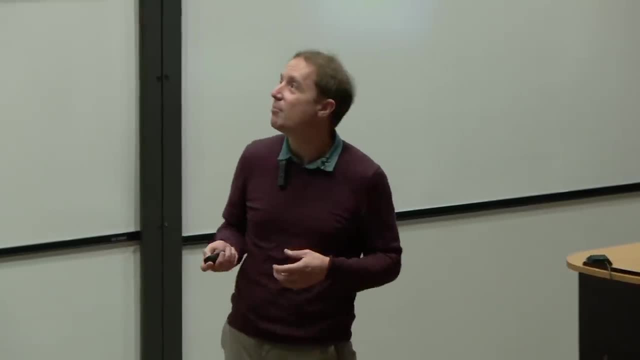 to my major point: What is it that applied mathematicians have got In all of these examples? we start with data, We start building up models And then we try and fit our models to data, And that's basically how we cycle through. 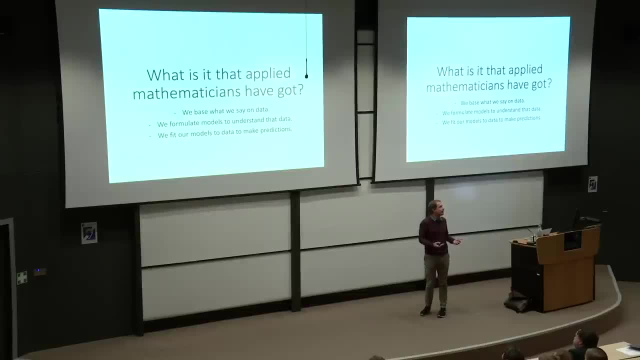 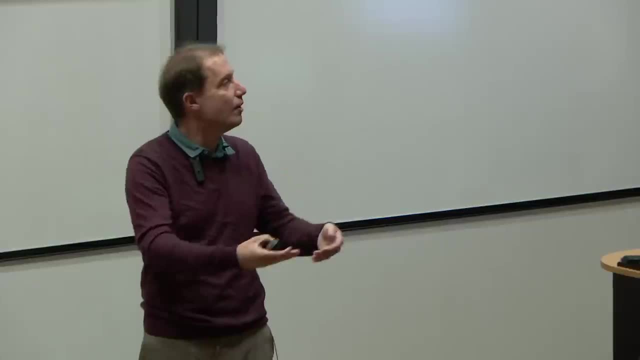 in everything that we do, All of the projects that we study are based on data, And that's the way we try, and then we try and fit our models to data, And that's basically how we cycle through in everything that we do, All of the projects. 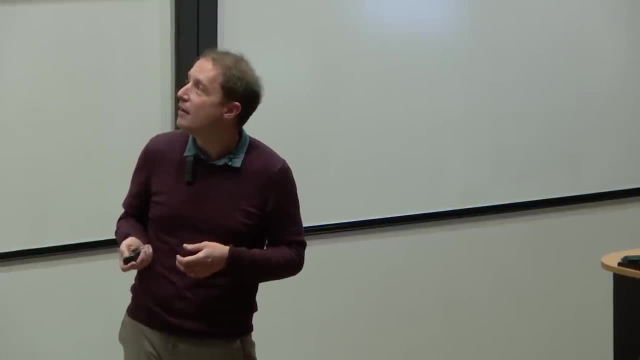 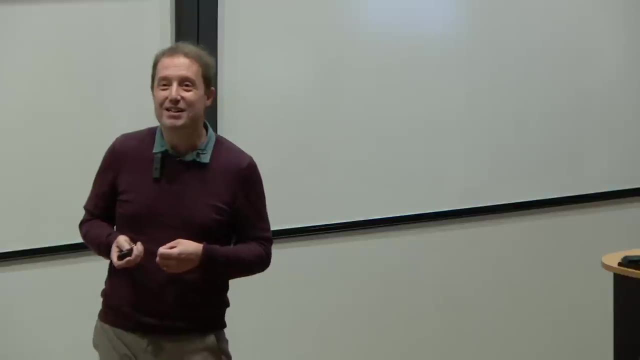 that we study are based on data, So we're not just- And that's really what I think makes applied mathematicians quite special- And we have got one very special applied mathematician here, And I learned- I myself learned- a lot of this art from Philip. 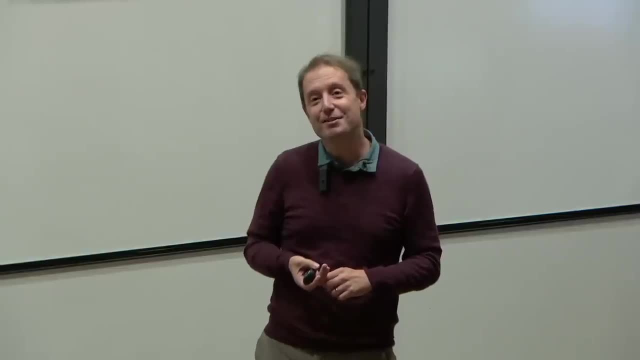 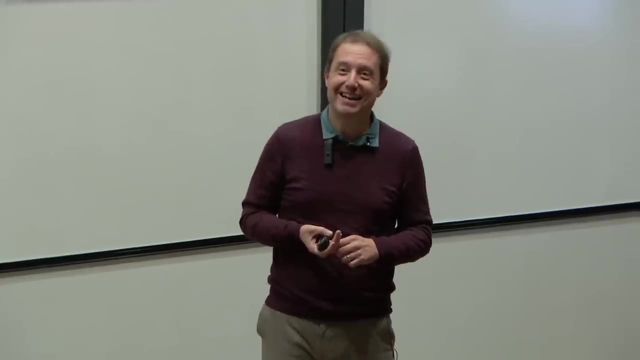 And I heard a rumor, Philip, that you have actually written to Premier League clubs and said: you've lost your or you know you've sacked your manager. You need a new manager And you have a collection of. you don't have any accepted letters. 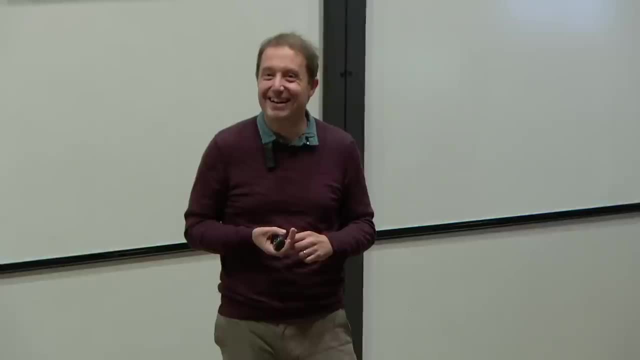 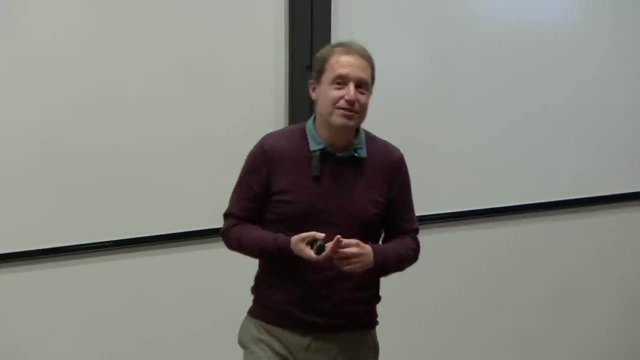 You have a collection of rejection letters. Is that correct? They're not rejection letters. They're considering my application. Oh, they're considering your. okay, Well, I think if anyone would like to pose a question, we can ask Philip about the contents of some of these letters afterwards.